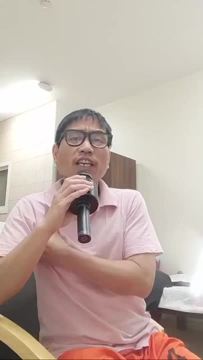 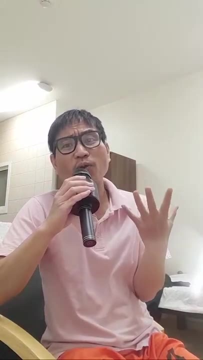 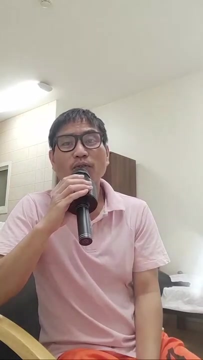 Now it's about time to touch in chemical engineering. okay, Topics and subjects. As you can notice when I go along with the discussion, it could not be denied that some basic foundations came from also from the physics and chemistry- again, really. 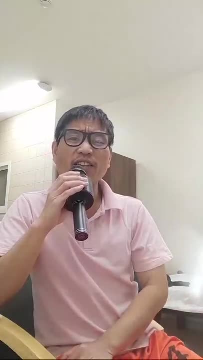 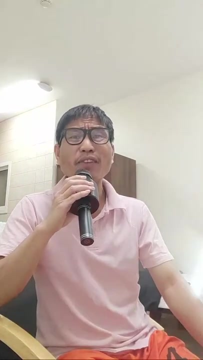 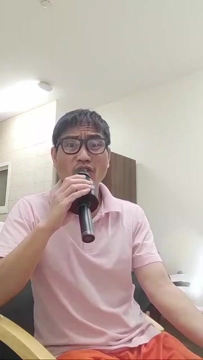 There's only an additional, okay, that focus on the complexity of the equations and formulas and a combination- you know, sometimes it could not be denied, sometimes calculus, sometimes differential equation, but not really that complex, only having an application. 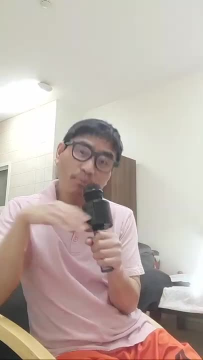 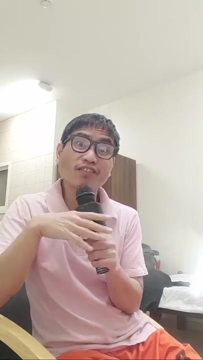 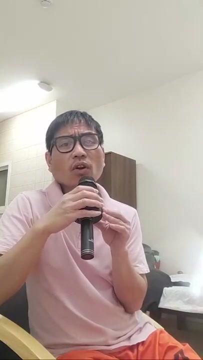 But in that kind of mathematics, okay, But still algebra will be there, trigonometry, something like that, but application only for the scientific laws involved in chemical engineering. okay, guys, So in chemical engineering we studied a lot also. 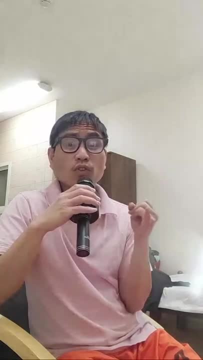 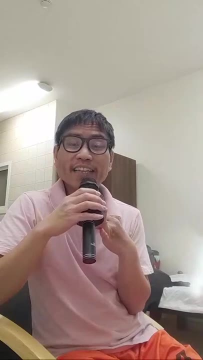 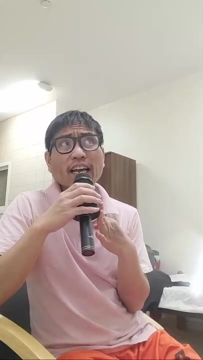 We have, I think, the industrial process control. okay, Number two: we have the chemical process industries, something like that, right, The stoichiometry. Number three, the chemical engineering calculations, something like that. We have the unit operations one, two and three. 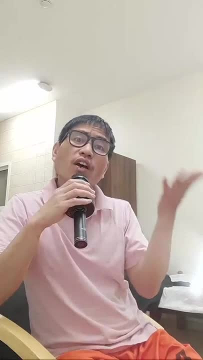 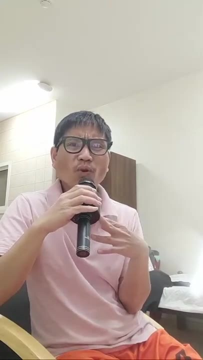 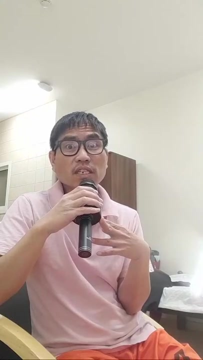 But this unit operations one, two and three, for example, the unit operations one composed a lot of the peaks. As I remembered unit one, we tackled more on the screening process. It talks about conveying systems of bulky solids. okay, 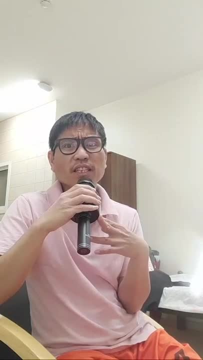 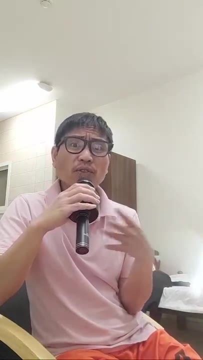 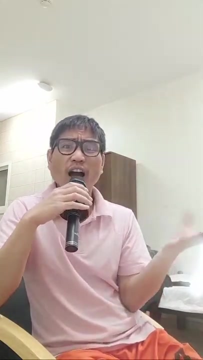 Something like that Screen- It's being tackled there- the size- particles of sand minerals or whatever, something like that to be screened, Talking about particles as diameters, something like that. okay, Aperture, mesh, mesh, mesh screening, like that okay. 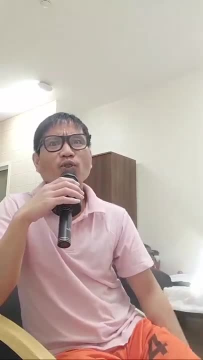 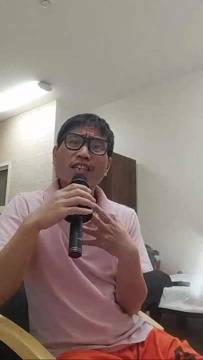 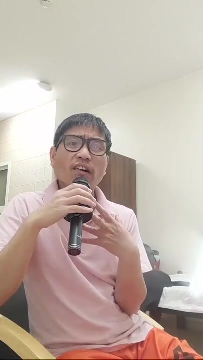 The diameter of the mesh, like that. It's all about unit one, okay. Unit two is more on the- Okay, I think so. More on the transport phenomena, okay. More on, shall we say, the momentum transfer, okay. 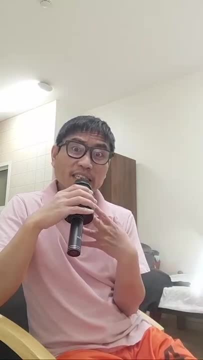 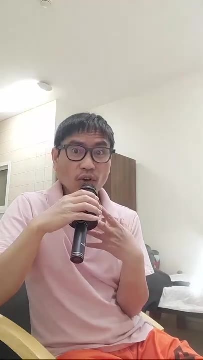 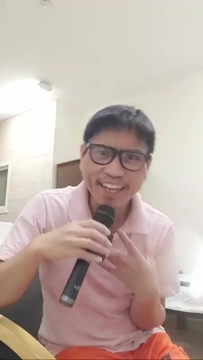 The fluid flow, okay, The fluid dynamics, something like that. Okay, The momentum transfer. of course We have the heat transfer through convection. We have also the- what do you call this one? Evaporation, something like that. 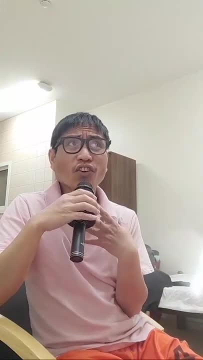 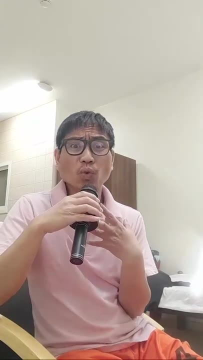 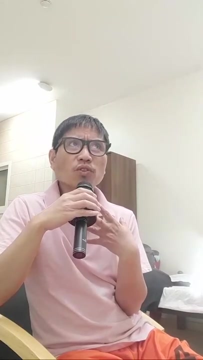 Okay, And I think filtration, crystallization, drying, flotation, leaching are also in unit two. Okay, And then unit three is more on physical and chemical separation processes. That's really it. Those are distillation, something like that. 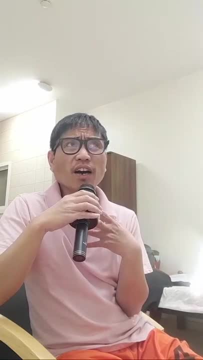 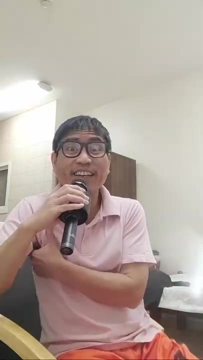 Okay, Distillation, And then the- That's it. A lot of physical and chemical separation processes, really Drying Like that. Crystallization, Okay. Chromatography: Okay, It's all about separation. Liquid-liquid mixture. 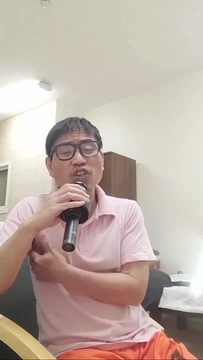 Solid-liquid mixture, Gas-liquid mixture, Gas-gas mixture, Something like that. Somewhere along the way we will also apply the thermodynamics for that. In fact, the chemistry, physical chemistry, is the combination of all. We will be applying that in the subjects for unit operations. 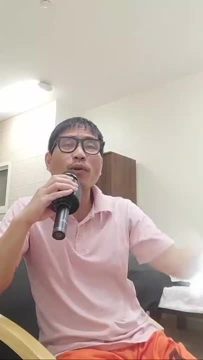 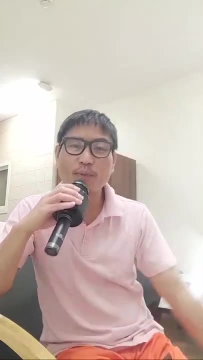 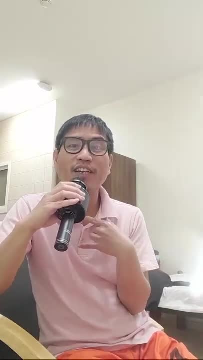 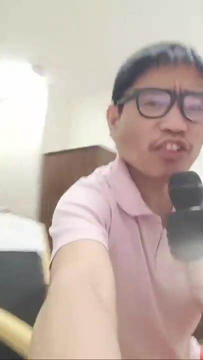 Thank you, Thank you. I want to remind you that if you do not apply the thermodynamics to any of the subjects, you will never pass the subject. You will never. you cannot take major chemical engineering subjects. Okay, Guys, I don't have to take a longer time. I guess vlogging or other topic. 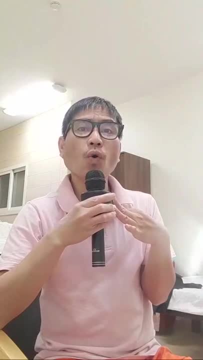 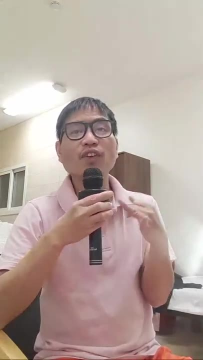 I hope you learned more about chromatography. Again, the first four separation processes that I will be able to discuss are okay: destilation, filtration, crystallization, chromatography- okay. And disinfect- Okay. Let's do that one by one. 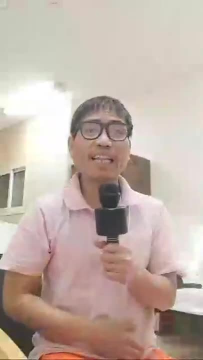 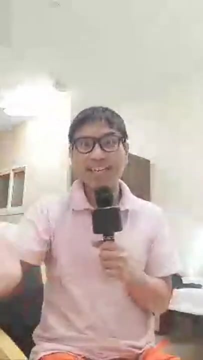 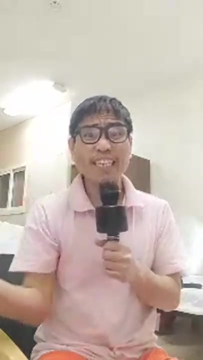 And after this for another physical separation processes. Actually there's a lot And it will never finish for three months. Instead, it is in detail, Something like that: There's a lot for the physical and chemical separation processes, The refining, the pyrolysis, the catalytic cracking, the thermal cracking, something like that. 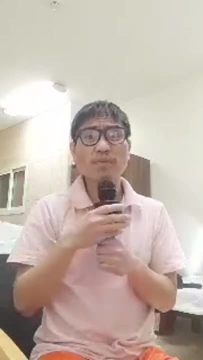 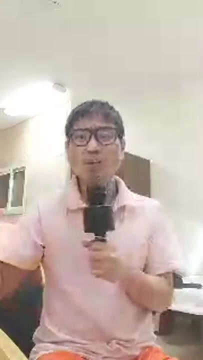 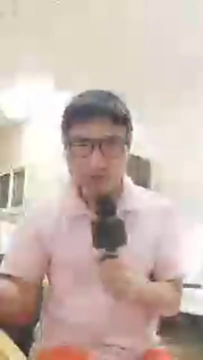 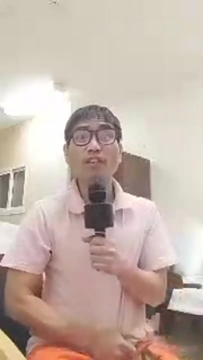 The desalination process, Okay, And then the polymerization process, also Okay. From large molecules to another large large molecules, From large molecules to lower molecules or smaller molecules, Something like that. Okay, And then the most popular in this topic is the petroleum industry. Really, Crude oil refining is the best example for this chemical separation process, Because it involves a lot- Okay, Not Not only the heating, the boiling and the desalination- It's always applied, the I mean Either it could be a physical or chemical changes. 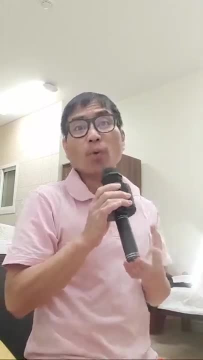 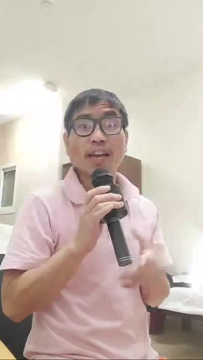 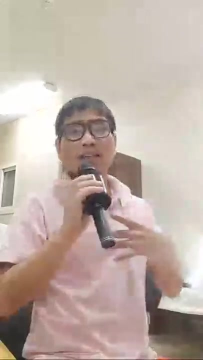 Okay, In this situation, you will remember always the mixtures, Mixtures And solutions, Something like that. Could it be a? heterogeneous mixtures, Homogeneous mixtures? Of course, If you mix liquid to liquid, like that mixture is homogeneous, right. 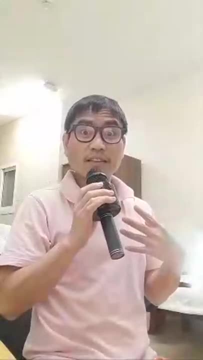 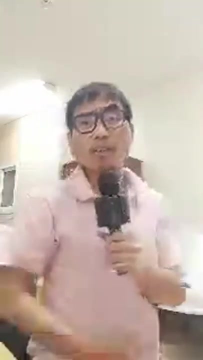 Liquid to gas mixture. So in this way, because you need to separate those phases one over the other, So we need to apply, you know, different processes for this. Okay, It could be also solid to solid liquid to liquid: chuba chuchu a lot. 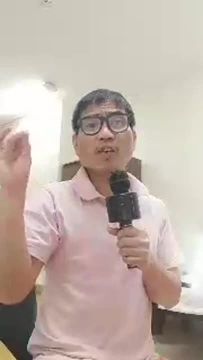 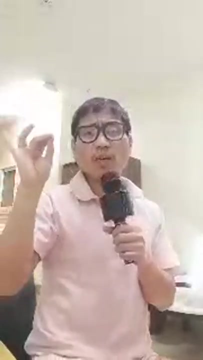 Okay, As long as you mix it, guys, solid liquid and gas- it's also going to be dry here, Okay, So the probability is going to be like that: Okay, Solid liquid gas. solid liquid gas, gas gas mixture. 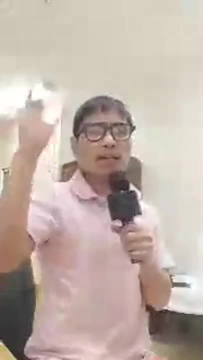 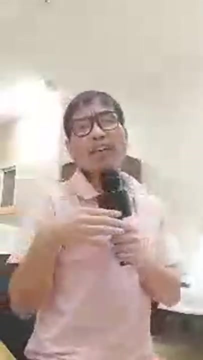 Liquid liquid mixture, Liquid gas mixture, Solid liquid mixture, And then applying the topic per topic, something like that, Okay, You get the point. And then some also are interconnected with each other. First you do the crystallization. 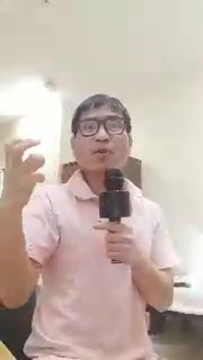 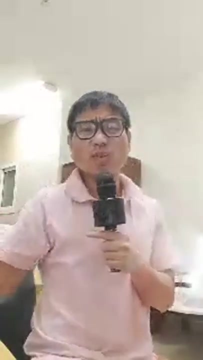 And after that you dry it. Okay, There's also process that involves a lot, from distillation, from heat, The crystallization, the last will be drying, something like that. Yes, Come back. This is again. I am a singer. eternal voice. 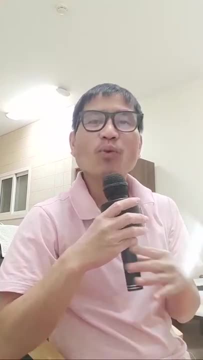 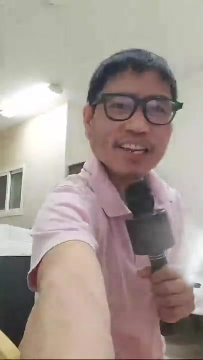 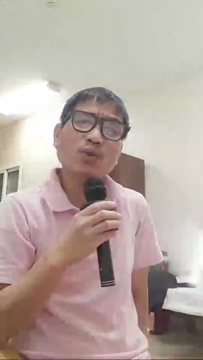 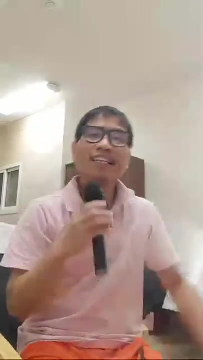 Welcome to the Science of Lama. At this time, we'll be able to talk about specifically chemical engineering topics. Okay, And now again, as I mentioned, awareness. We need to tackle The, you know, the distillation. okay, first half and then okay, gradual discussion. 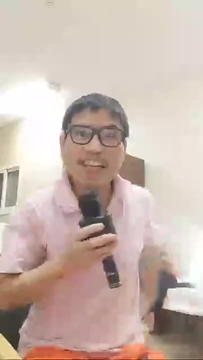 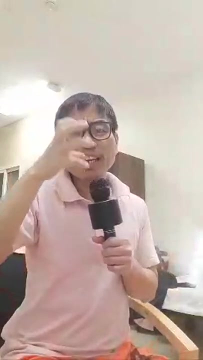 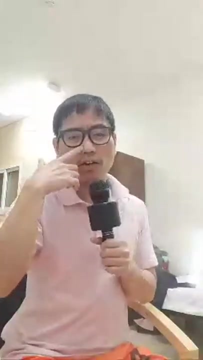 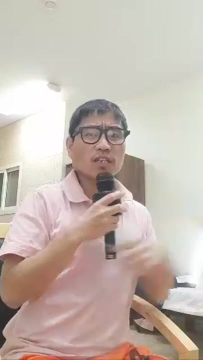 of the topic. okay, We don't know really the comprehensive. you know topics and knowledge out of it or learning out of it. okay, So distillation. So distillation what? What do you understand for this physical process? okay, 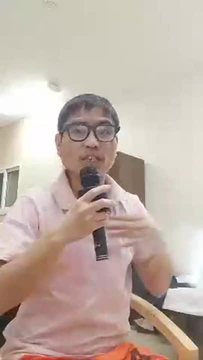 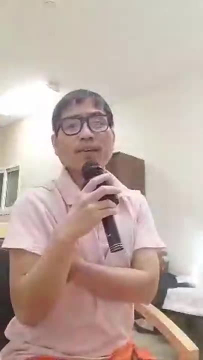 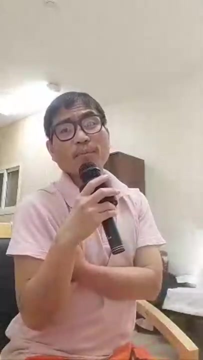 This is not a chemical process, This is a physical process. okay, Any idea? Okay, I will be the one to answer. of course, I will be the one to discuss. okay, Distillation is a physical process that is used to separate mixtures. 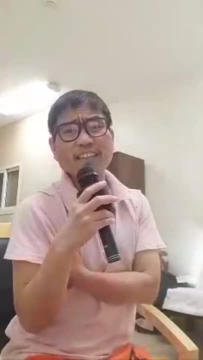 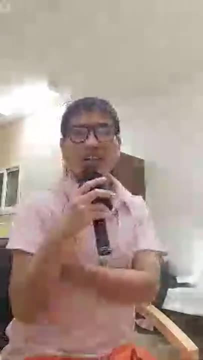 Could either be liquid-liquid, solid-cast, something like that, based on the difference of their volatilities And boiling points. okay, Boiling points. So it's in here that we need to. oh, so what's volatility all about? 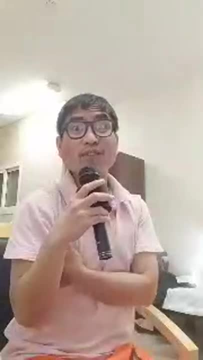 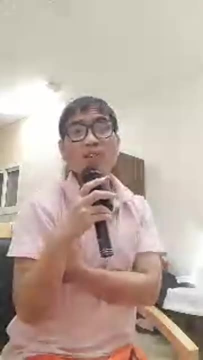 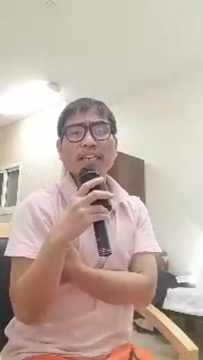 And what is boiling points So that we can understand really what I'm talking. in the definition alone, Okay, When we speak about volatility, it is a physical property or a characteristic of a liquid or a solvent that could easily vaporize into atmosphere, meaning to say it will vaporize. 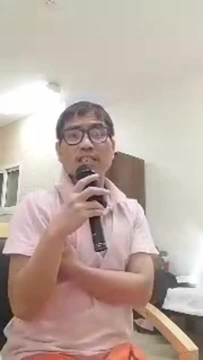 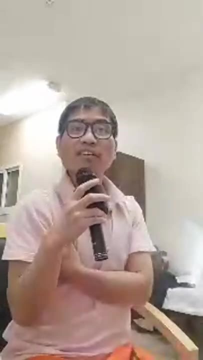 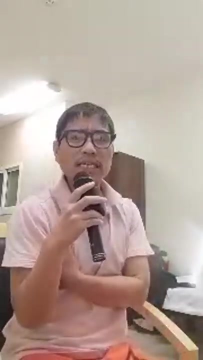 change, Change into vapor from a liquid, the ability of that certain liquid substance to anergo. volatilization- right, Because it's a process. volatilization- okay, That's volatility. For example, if I put water in front of me and then I will on my AC, or even though 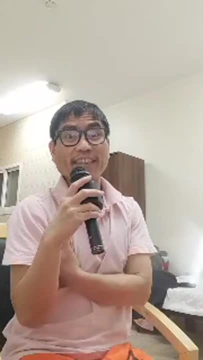 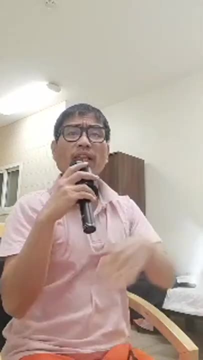 it's your AC and there's a hot environment, something like that, so there will be a heat transfer. So time will come that the liquid will vaporize. The liquid water will reduce the volume slowly, slowly, slowly, slowly, slowly, slowly, slowly. 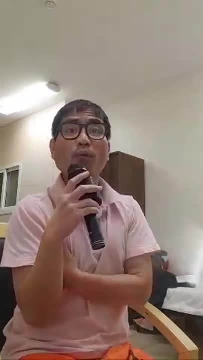 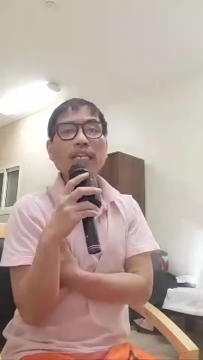 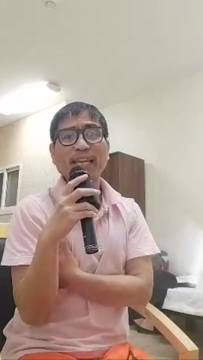 because water has its volatility physical property, just like other solvent also. okay, It will vaporize in the atmosphere, naturally, meaning to say, without inserting, adding or without the application of energy, anything, you don't touch anything, or whatever. okay, 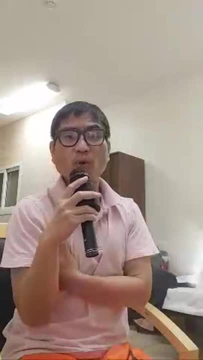 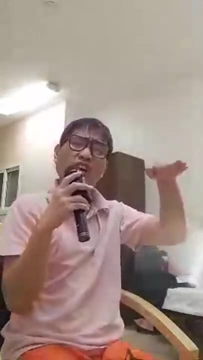 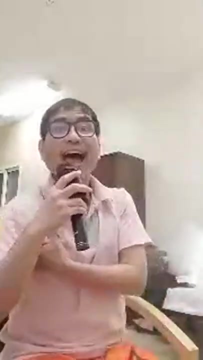 This is a natural process. This is spontaneous process. okay, You don't have to do anything. It will just lower down a bit the volume until such time it will be reducing until all will be evaporated into atmosphere. So those liquid substances has the volatility characteristic, okay. 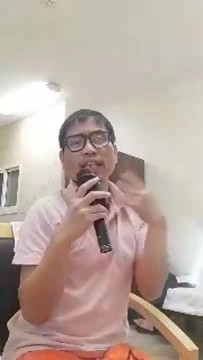 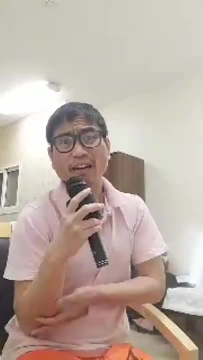 Like that. So we said, ah, volatile, non-volatile, non-volatile, there's no chance to. you know vaporize, you know vaporize in the atmosphere, something like that, if you don't add water or anything. 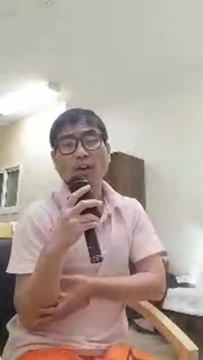 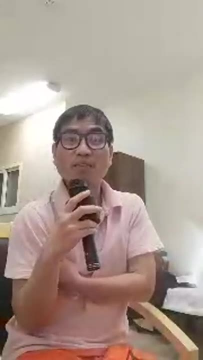 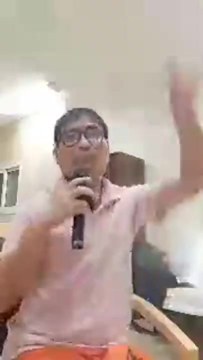 okay, Just like sodium chloride, it will never create vaporization if you will never add water to the salt. okay, Because that is a non-volatile solute. okay, But it will lower the vapor pressure of the solution. it will never be escaping to the 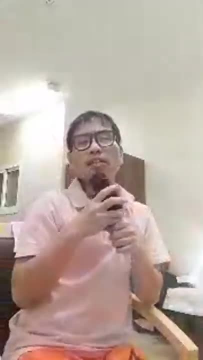 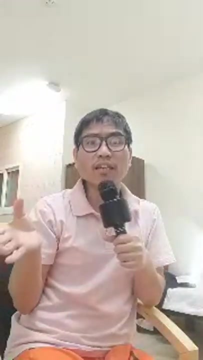 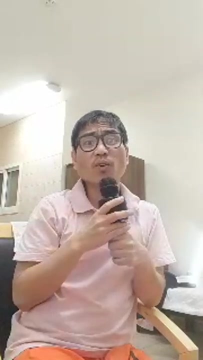 atmosphere without the addition of a solvent or a liquid. okay, So that's volatility characteristic. Now we go to the boiling point. What do you mean by boiling point? Okay, the key term here is boiling. okay, Of course, when you boil a substance that's normally liquid, okay, 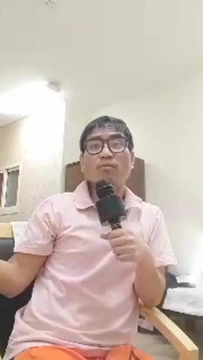 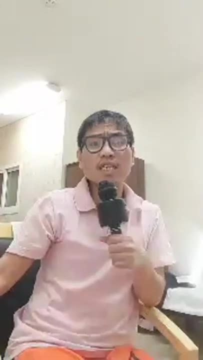 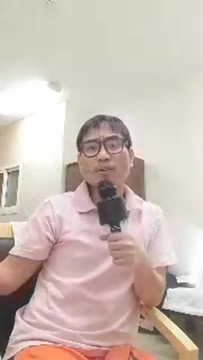 Then if you just heat the solid, that's not called boiling because it's not liquid Meaning. if you say boiling, guys, it refers to liquid or solid and a liquid. But you know you will never say technically that if you heat, for example, the sodium, 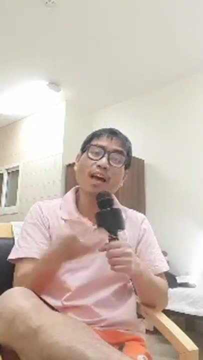 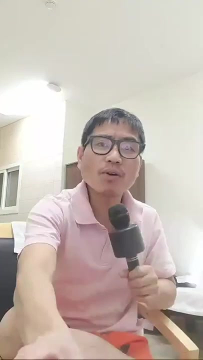 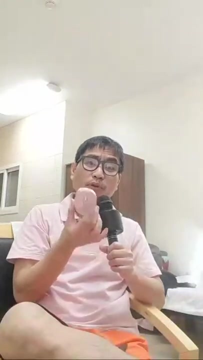 chloride, that's boiling solvents. okay, The you know the application of terminology. okay, For example, I have a plastic, I have a glass here and I will try to burn this one at a certain temperature so I'll be able to burn. 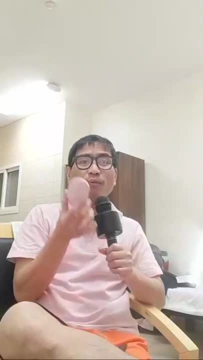 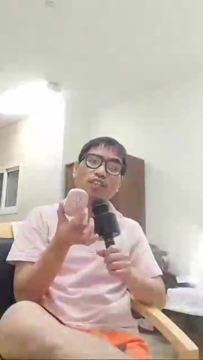 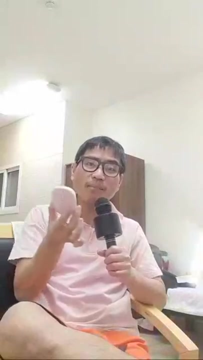 So meaning to say I do a pyrolysis physical process. Pyrolysis is the act of burning objects or substances at certain high temperature. for example, okay, I will not say I will boil this mouse. I will say I will heat this mouse on my laptop so that this will melt. okay. 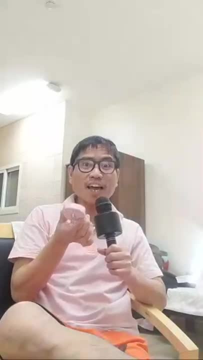 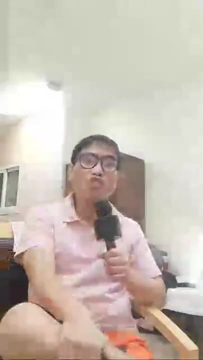 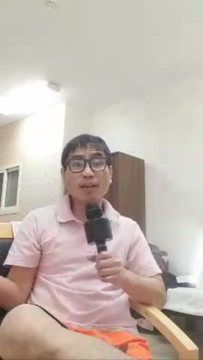 Something like that. So this will undergo a melting point after boiling, after heating. Boiling is not the right term. It's applicable only for solvent and liquid. okay, If I have the alcohol here, I will say I will boil this alcohol to a certain boiling point. 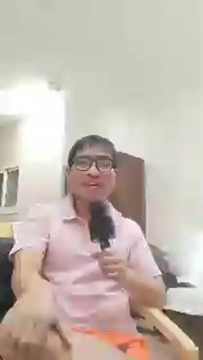 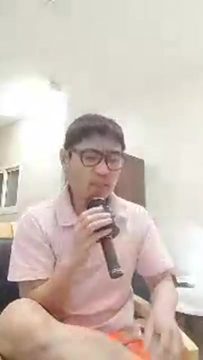 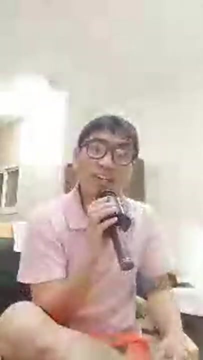 something like that. okay, So that's correct, You get the limitation. but heat is all solid liquid like this, okay. And the boiling point- really guys the definition for that is when the vapor pressure of the liquid- okay- will be equal to the pressure of the liquid surrounding. 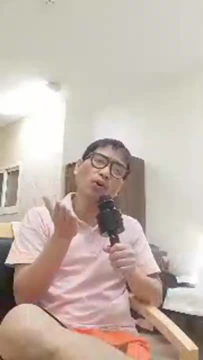 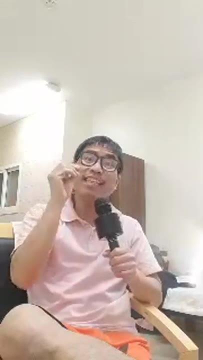 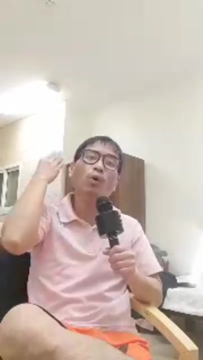 Get the point Meaning to say, for example, if I put water in a kettle, the you know, the pressure of the vapor will be the gas, okay, The molecules of the vapor. it has the pressure When that pressure exists, or achieved, if it will, in equilibrium to the pressure of. 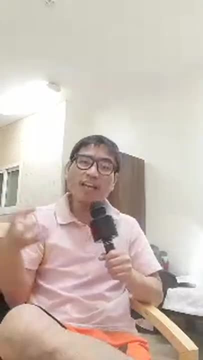 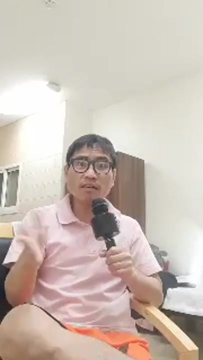 the liquid surrounding, the surrounding of the liquid. now that attains boiling point. If it will never equal pa siya, then it will never boil. okay, So normally water at 100 degrees Celsius, but for higher molecular weight compound. 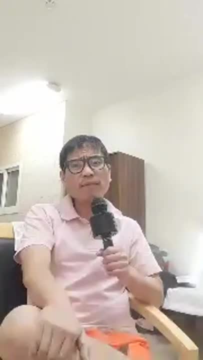 it will be lesser, okay, Something like that. okay, You get the point. Boiling point: boiling point is dependent to the molecular weight. okay, Okay, Did I say it correctly? Okay, I'm sorry. If it has a high molecular weight, the boiling point is very high. 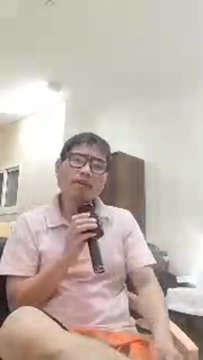 Oh my gosh, Sorry po, it was corrected in the brain cells. okay, Okay, Ako di-analyze kung bu-ak siya Baglay sun ka bu-ak. Okay, Okay, Okay, Okay, Okay. 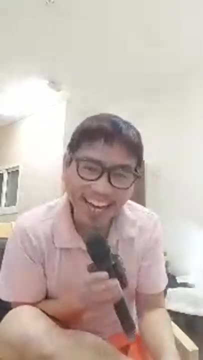 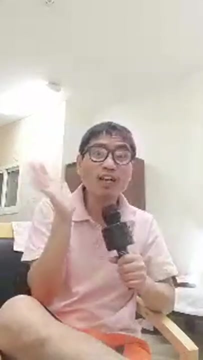 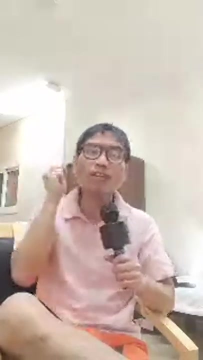 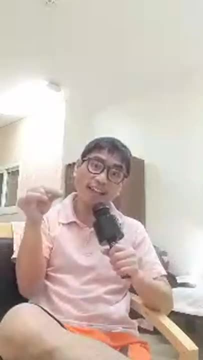 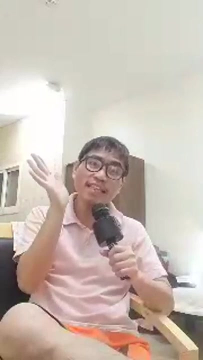 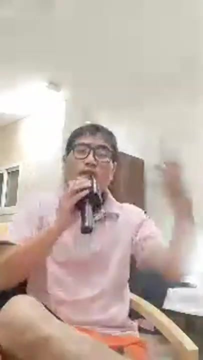 Now, since you heat, that heat means heat energy, it's just the same. okay, When you heat, you apply energy, of course, and that is heat or thermal energy, and then it will develop the kinetic energy for that, because the molecules will be in motion, bombarded. 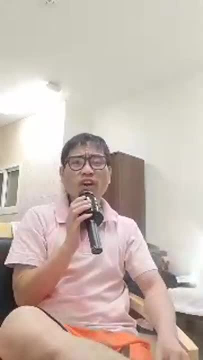 with each other To obtain the strong intermolecular forces to break the bonding, the chemical bonding of a certain liquid, something like that. But for molecular, with high, high molecular weight, it needs too much temperature or heating process compared to the low boiling point. 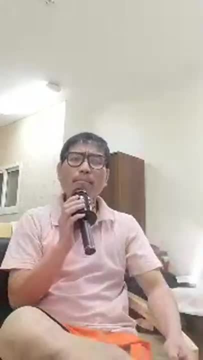 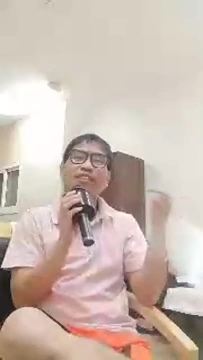 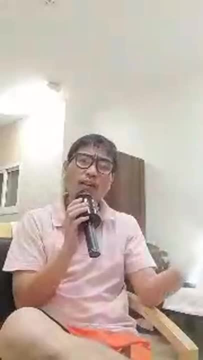 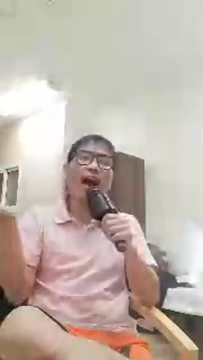 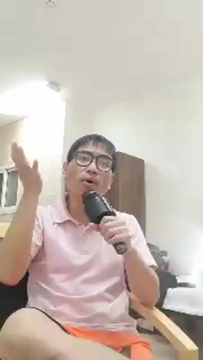 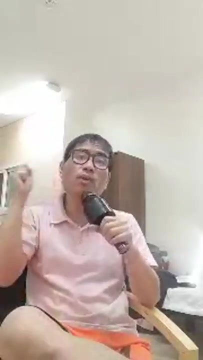 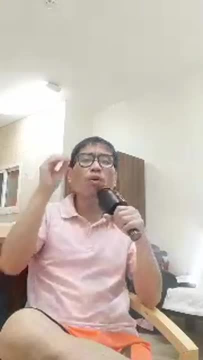 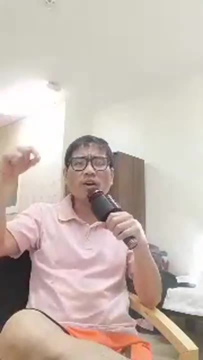 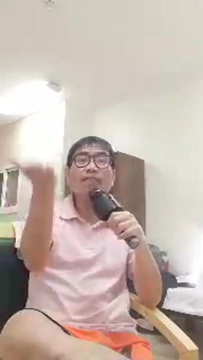 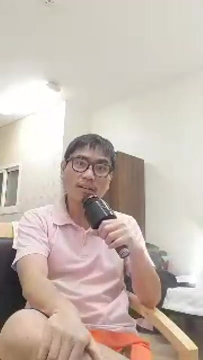 Okay, Okay, Your bacteriognosmosmojniosm- artificial buckles. Okay, All right, Now Today. molecular weight, then. if the molecular rate is high, then automatically, without referring the group that is having a high boiling point. okay, then the question also will say which of the 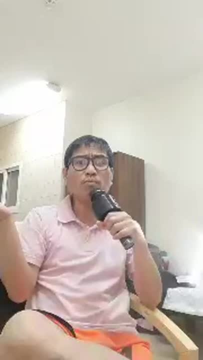 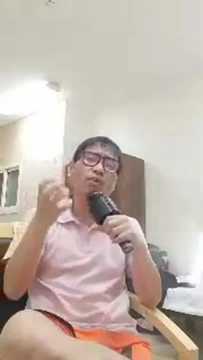 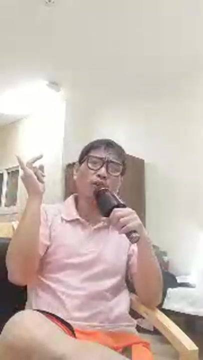 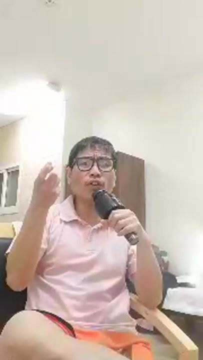 following: needs high kinetic energy. okay to boil, then choose also the one that is having a high molecular weight, because molecular weight is directly proportional to the kinetic energy, directly proportional to the heat energy, directly proportional to the activation energy and directly proportional to the intermolecular forces. I enter molecular IMF, intermolecular. 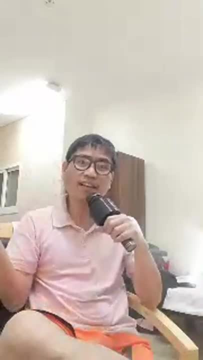 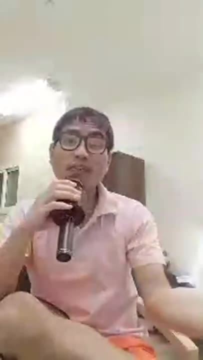 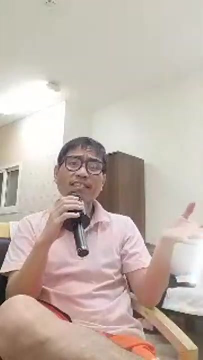 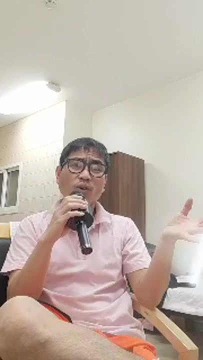 forces- okay, the two points, something like that. the molecules- okay, okay, okay. whereas the gas, the molecules distance are very far with each other, so you don't have to put extra heat for that in order to boil right to be there for us, the liquid, the molecules are. 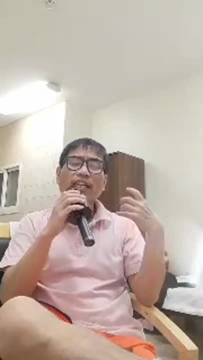 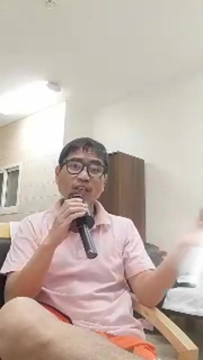 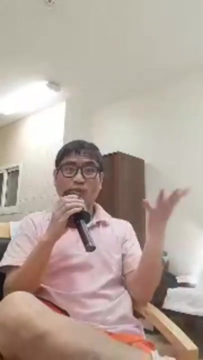 something closer with each other than shop. so it needs heating more compared to the gas. so we need to say, guys, gas has a higher volatility to liquid compared to liquid. you got the point, okay. and then this gas, of course, vapor na siya. eh, so dala na kayo siya i-boil, okay. so gas or 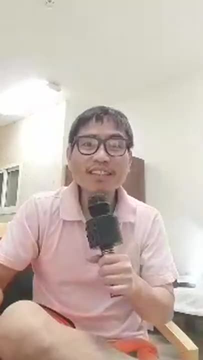 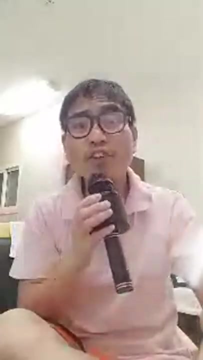 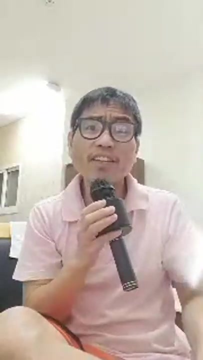 vapors have a higher boiling point. of course, common sense diba okay, ganun siya. okay, so that is volatility and boiling point. so the boiling point of water guys is 100 degrees Celsius. okay, that's the point. so it depends on the molecular weight. okay, you can determine if 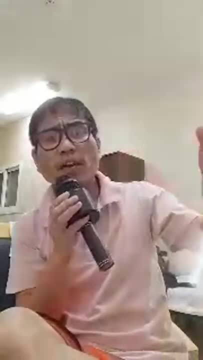 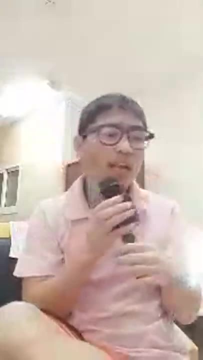 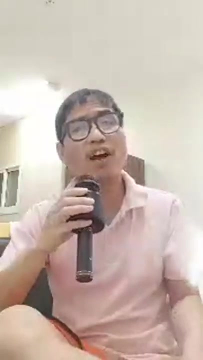 it's high boiling point or low boiling points, okay, but we separate these liquids to liquids in based on the boiling points. is distillation okay now? oh my gosh. in distillation guys, it involves two processes. what are this? you can never have distillation without these two physical properties: processes. 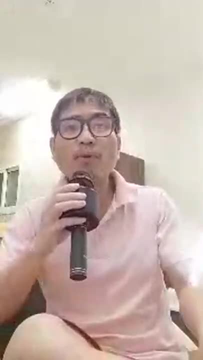 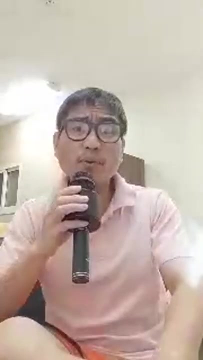 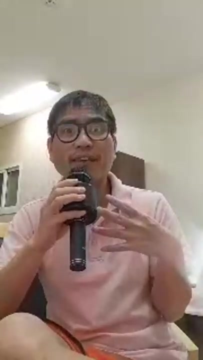 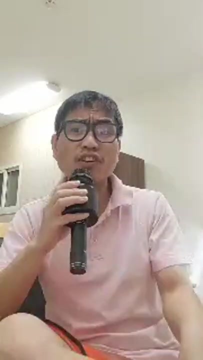 so these are evaporation or vaporization and condensation. okay, what do we mean by evaporation and vaporization? okay, I'm just reviewing the chemistry in high school or elementary level. okay, this is, this is Elementary science. okay, what do you mean by evaporation and the transition? a? 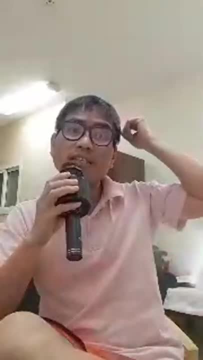 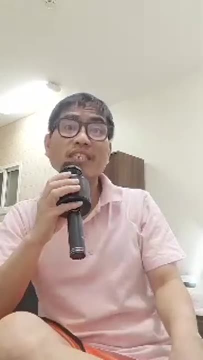 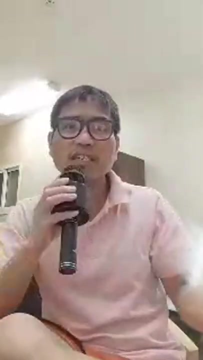 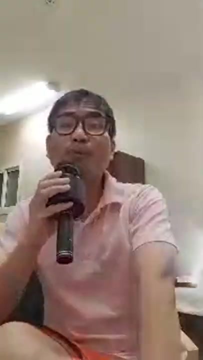 change from liquid to gas. what we mean of gas, guys, that is technically vapor, because gas that is in a vapor state in the atmosphere, air mixture in our environment, something like that. okay, so that's the polarization, so meaning to say the destination, guys, we need to evaporate, evaporate. we need to evaporate the liquid to 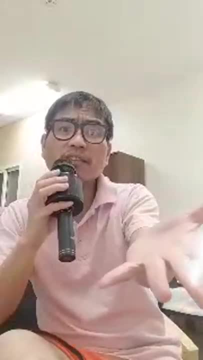 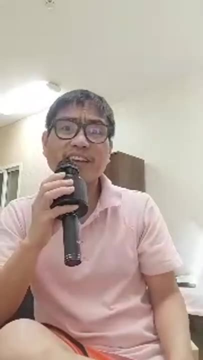 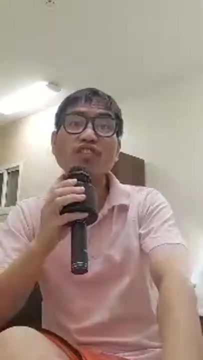 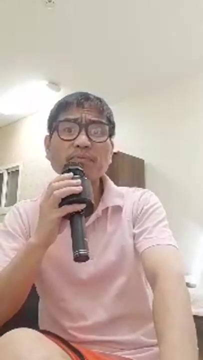 produce? to produce what? distillate or condensate? to produce a condensate, not distillate guys. to produce a condensate by heating and boiling. okay, that's why we have condenser in our distinction column. the purpose of that is to condense something like that. okay, so the condensate will be produced. 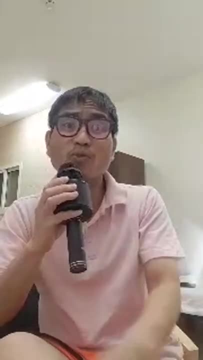 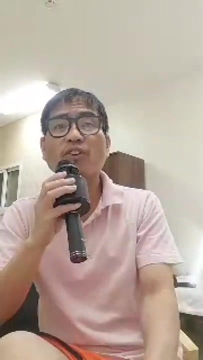 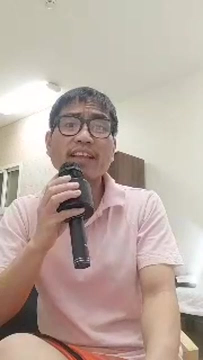 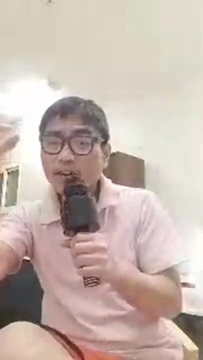 okay, sometimes it takes confusion. supposedly that is condensation, right, because we produce condensate. but believe you guys, okay, electrochemical or electrochemistry, that our is positive terminal, our cathode is a negative terminal because it is where the cathode will react, there okay, in that particular terminal. something like that here also reverse, okay. 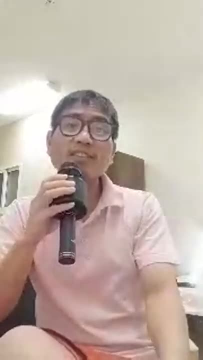 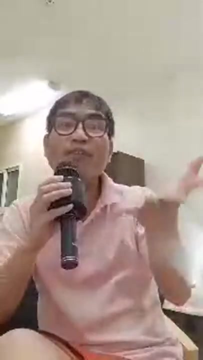 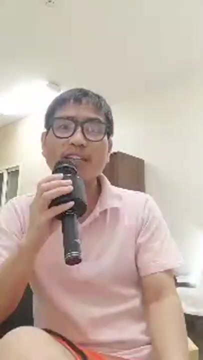 supposedly this will be distillate, right, but it's not. it's condensate, okay. and the second process is: we need to condense the, the vapor. we need to condense the vapor to produce a distillate. you get the point. this is meaning liquid product. bear this in your mind. the 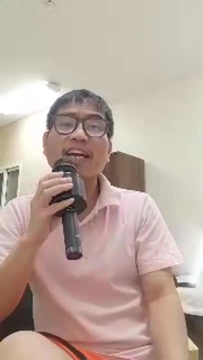 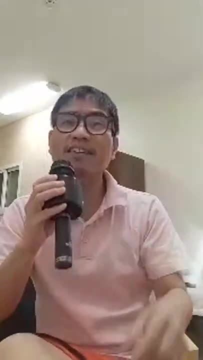 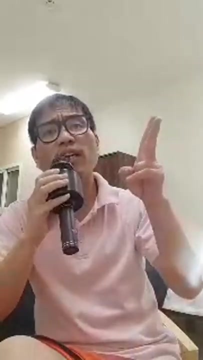 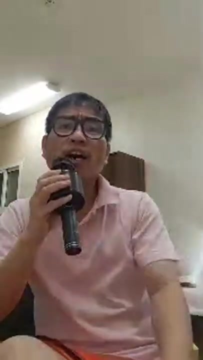 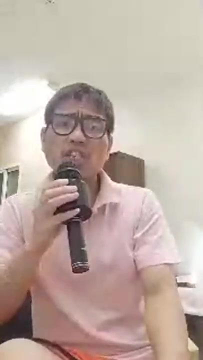 distillate is a liquid product. the condensate is a vapor product. okay, so distillate is a liquid product by this time. by cooling process. okay, so heating cooling will be applied there specifically. okay, but these are under evaporation and condensation respectively, so we can say that condensation. 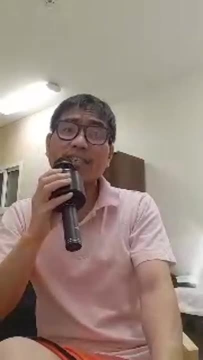 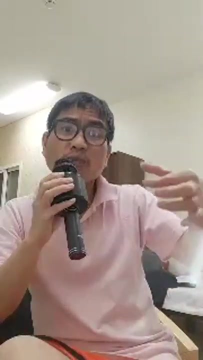 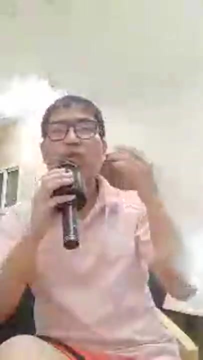 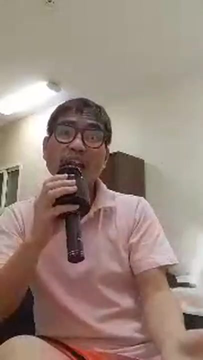 is a phase change from gas to liquid. okay, because we say we need to condense the vapor before it's a gas. okay, and then to liquid, we have the distillate, like that, okay. so we should not be confused, because we'll be using the fractionation calculating how many number of trays, something like that in a. 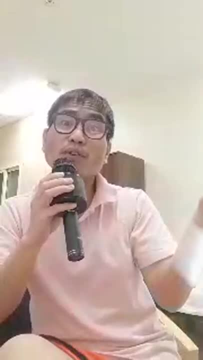 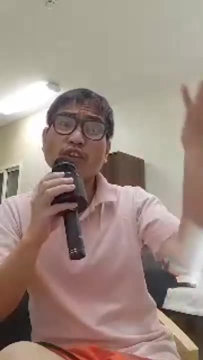 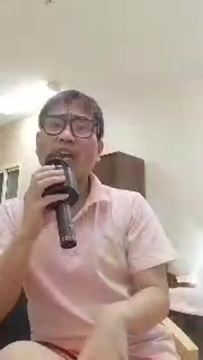 distillation columns multiple, you know multiple- number of traces by using the mccain field method in distillation. you need to hold it for the slope, something like that. the white intercept: okay, and the blood, so the feed, okay. the reflex, something like that, so okay, that will be more. 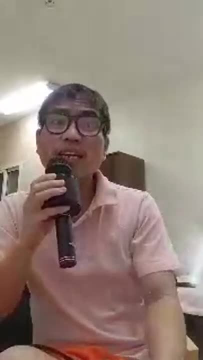 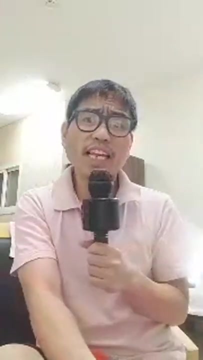 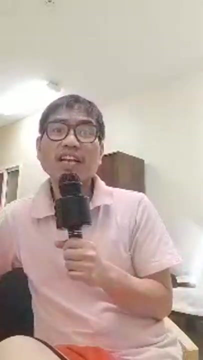 this is just an overview yet. okay, something like that. okay, so that is distillation. okay, guys, now we need to know the two types of distillation. only there are only two types, right, but actually there are a lot, but those are kinds of distillation, kinds. kinds and types are not the same. 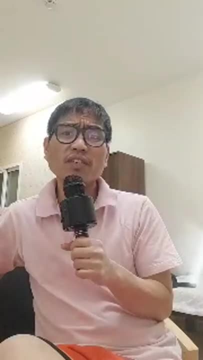 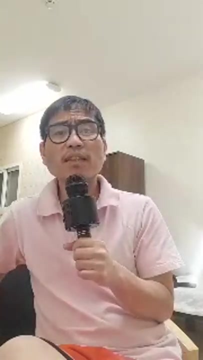 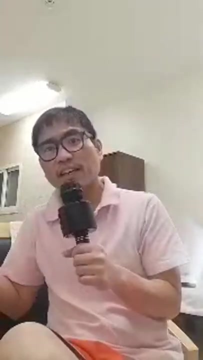 okay, types refers to the, the method, but the kinds refer to the materials of construction used for in equipment used. okay, like that. but the types are based on the method or the procedure. that is gonna be the way you do it. that's why it's called like this. so that's types p-y-p-e-s, but kinds a lot. 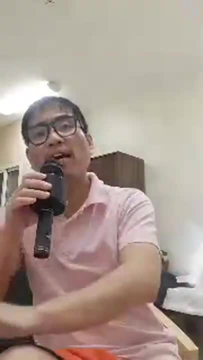 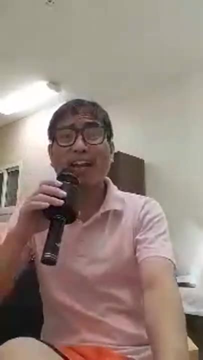 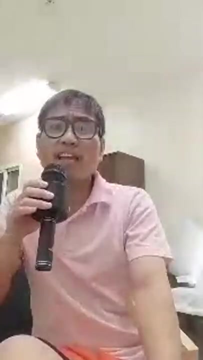 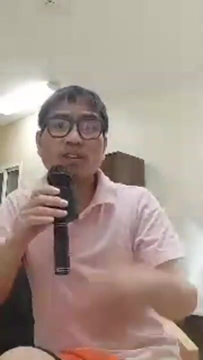 of kinds, for example, if i use this kind of blah blah blah and another also kind of material, but producing the same purpose. so that are kind the values. kinds of molecules, types of molecules okay, types of molecule, large and small, molecules okay, and then for kinds, a lot, there's a lot of. 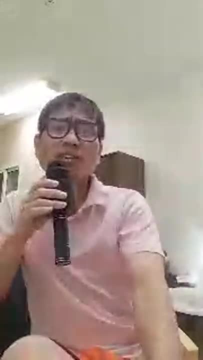 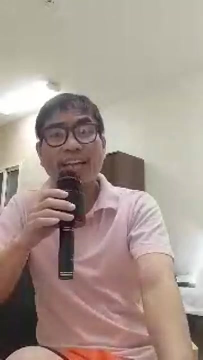 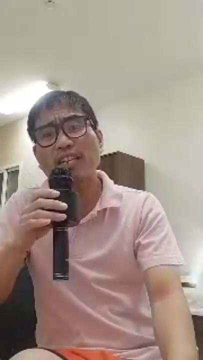 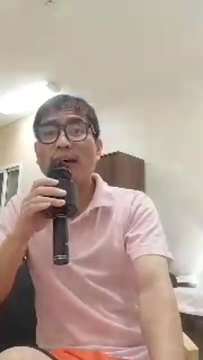 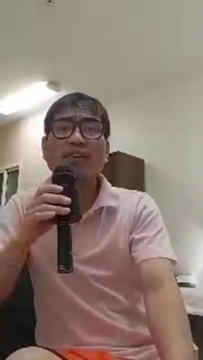 kinds. you have the organic, organic, hydrophobic, hydrophilic substances. okay, you got the point. types of kinds of examination, classifications of blah blah blah. okay, what are the types of blah blah blah? what are the kinds of blah blah blah? and also the. you know the category and the class before. what are the? 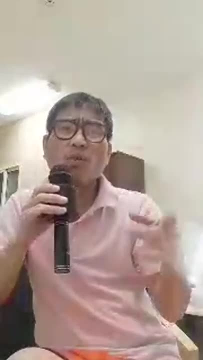 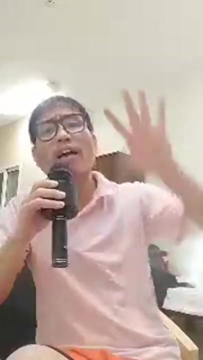 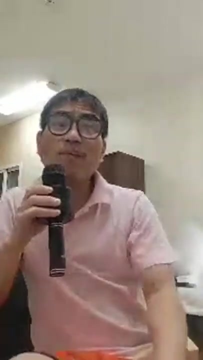 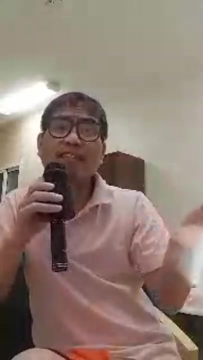 four types, classes of reaction. what are the four types of reaction? Ganoon, what are the four categories reaction? so what are the kinds of reaction? okay, in chemistry we have five types of chemical reaction. right, it's about the method. how do you do it, like decomposition, reaction, synthesis, combustion. 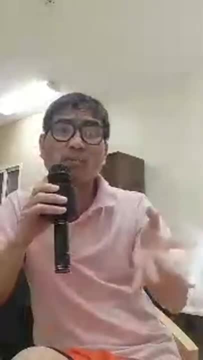 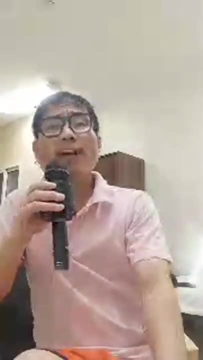 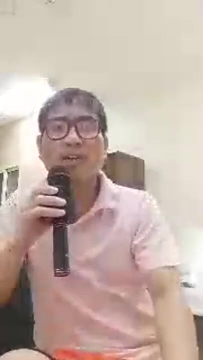 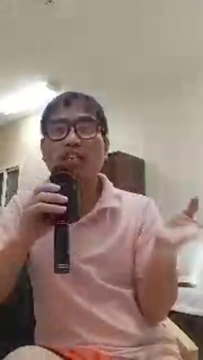 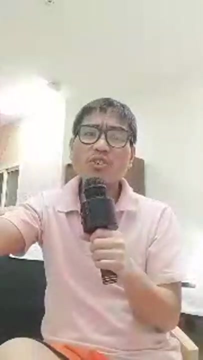 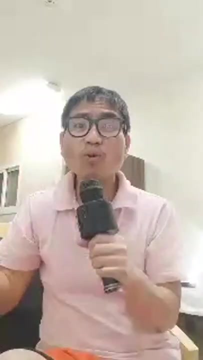 hydrolysis, neutralization reaction, double displacement, displacement replacement like that photosynthesis. but what are the kinds of chemical reaction? do how to get your guys irreversible reaction and reversible reaction? okay, during enumeration and list listing questions, what are the kinds of uh chemical reactions? would you try reversible chemical reaction and irreversible reaction? 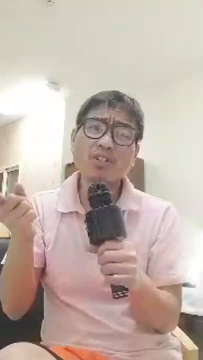 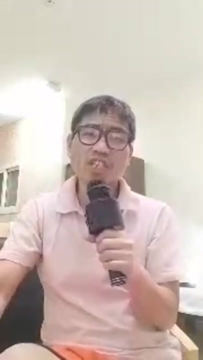 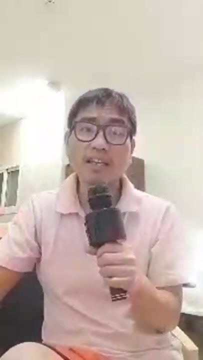 okay, or spontaneous chemical reaction or non-spontaneous chemical reaction. spontaneous chemical reaction meaning reversible reaction. non-spontaneous chemical reaction: irreversible reaction. it doesn't, goes back to its original state. okay, it is a powdery covenant voltmet. then it is resolution. one try地вод. 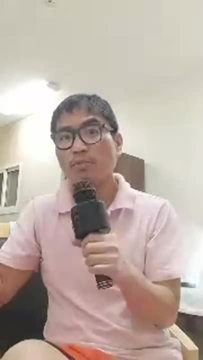 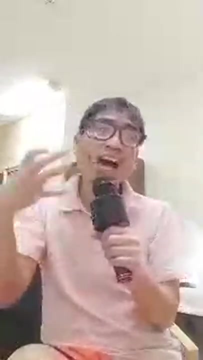 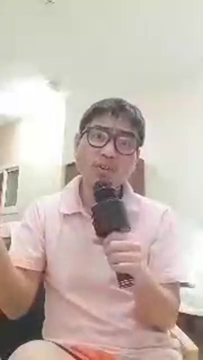 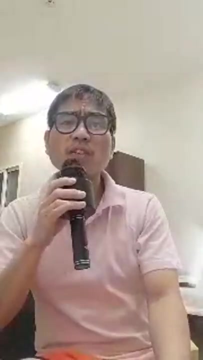 okay, it will just produce another byproduct, byproduct, byproduct, byproduct. but the reversible, spontaneous, it will, goes back to its original uh reactant without doing anything, without adding energies, without altering the composition. okay, without changing the parameters, naturally spontaneous. okay, so in your generation, because this spontaneous, non-continuous, 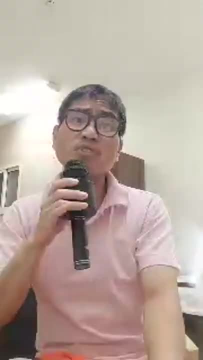 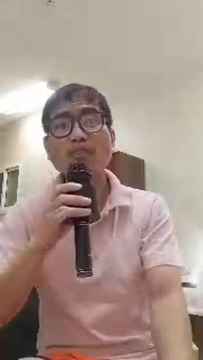 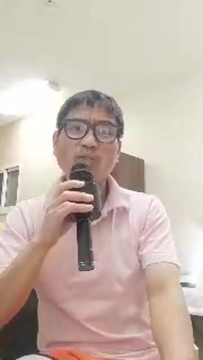 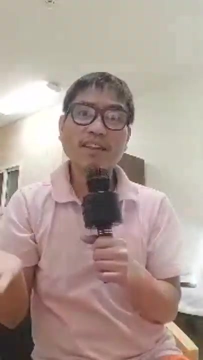 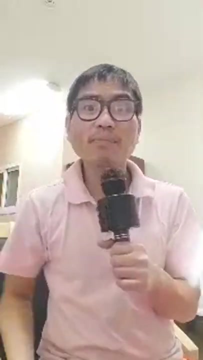 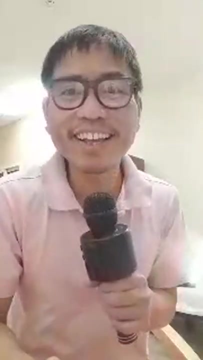 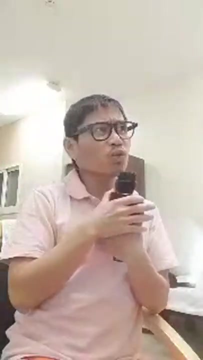 irreversible higher science subjects, uh, chemical engineering, physical chemistry, thermodynamics and unit operations classes: chemical reaction engineering or chemical reaction kinetics. okay, okay, so don't believe me. fundamentals, basic fundamentals and basic foundation, so that we can understand really mayabu. okay, you get the point. okay, so that's what we mean. okay, going back um two types of distillation: okay, 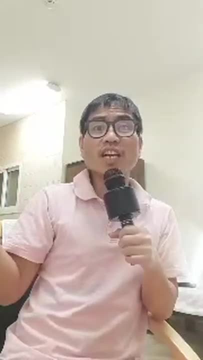 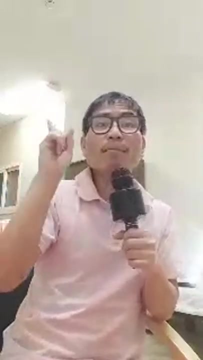 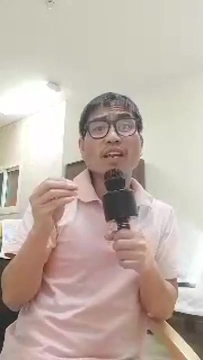 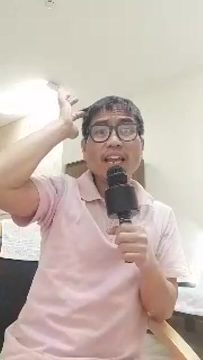 d-a-t-c-h: okay. the conventional distillation: okay, we have the simple destination and the fractional distillation. if we mean fractional destination, it involves a lot of definition, columns- okay. a lot of trays in the columns which are column units- okay. and then another is the simple destination, having only one. 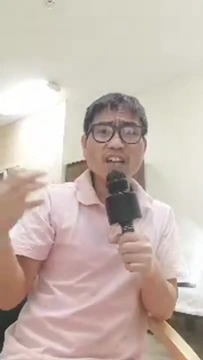 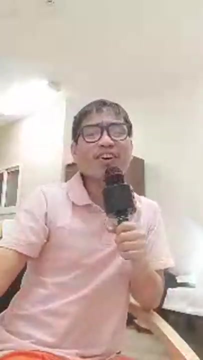 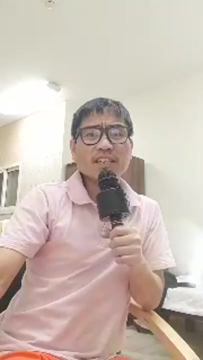 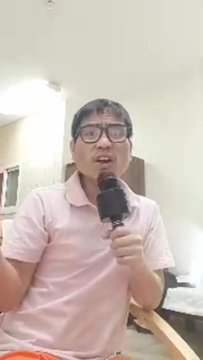 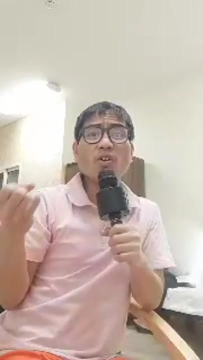 like that. there's no lot of trace, okay, so the simple destination there's just one. the whole processchas is this. it's the main function of distillation it in the sterile processch, processche, right, okay, what we we have now is that, like the series, 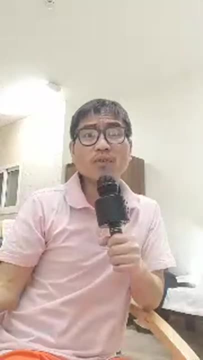 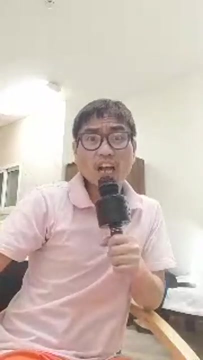 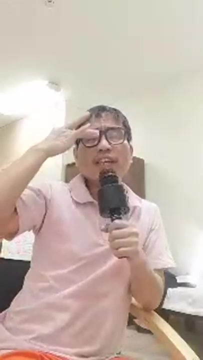 the sequence component is vaporized into the atmosphere and be collected as our condensate, something like that. okay, okay, okay, you get the point. and then in a distillation column, in a simple distillation guys, the, the liquid will flow downward and the vapor will go upward. common sense again. 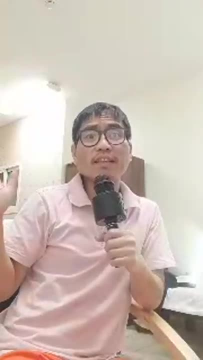 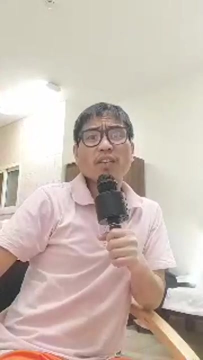 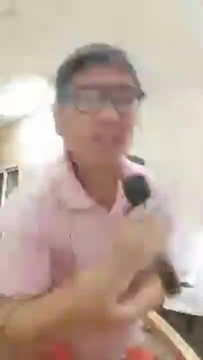 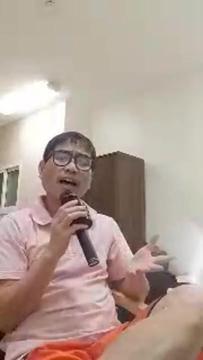 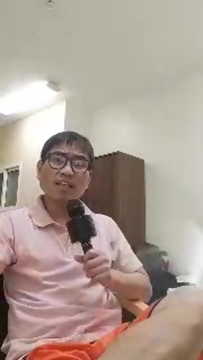 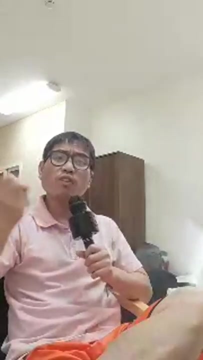 because vapor has lower molecular weight, low density compared to the water. okay, you get the point. the the more it will become wet, the more it is having a very high mass. okay, because the moisture is there. okay, the moisture will contribute also additional molecular weight to the liquid, uh, substance. but whereas the dry, only the, you know. 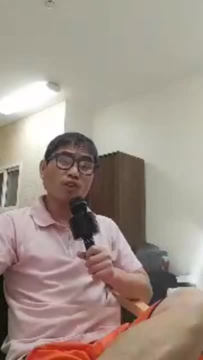 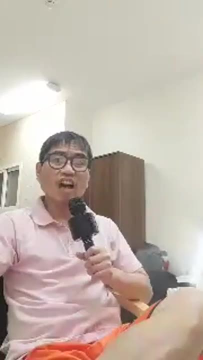 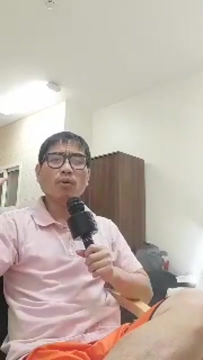 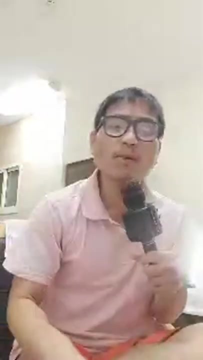 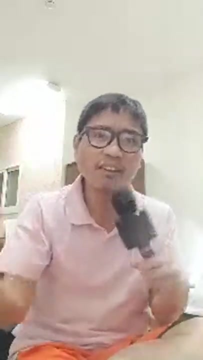 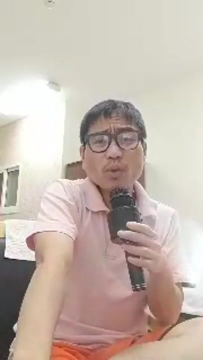 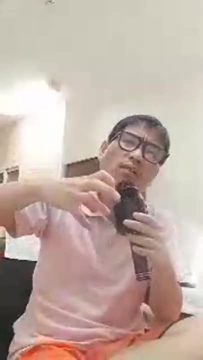 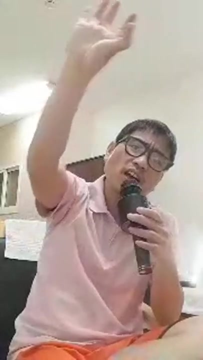 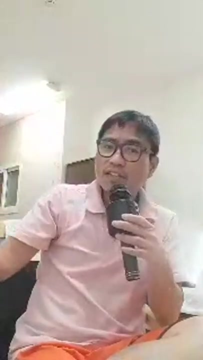 interesting in the liquid, for example, my distribution column, and we hit that at the bottom right like that, and then there's a thermometer at the top and there's a condenser there and inclined position attached to the distillation column and there's also a beaker somewhere in the right and 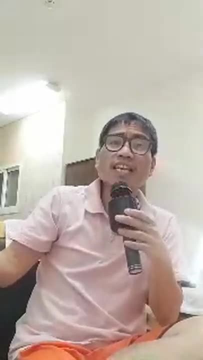 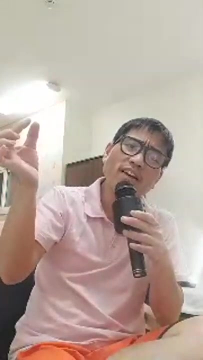 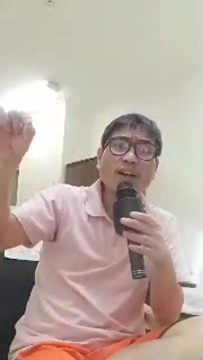 the beaker, what we call this, a sink to catch the distillates there. okay, this condenser have two outlets. the two outlets, guys, are the cooling motor that goes in into the condenser- okay, that will become our distillates, right, because the equipment shop. okay. and then the other one also. 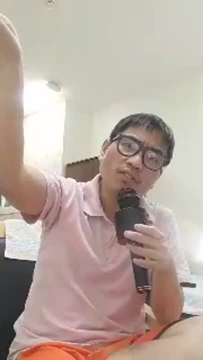 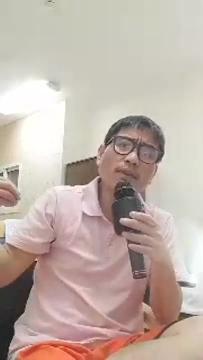 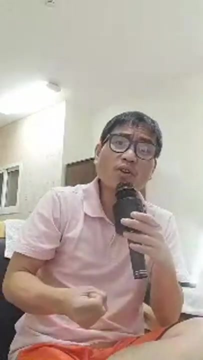 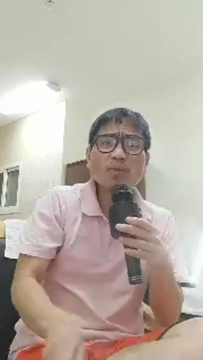 the other one is the: we will come out, the vapor will come out to the other hole, okay, something like that. so the liquid will come in, the vapor will come out, something like that. so meaning to say: parang steam, right, the steam will goes out. right, ala nga magtigo mo ng steam. okay, it will just goes out, okay. 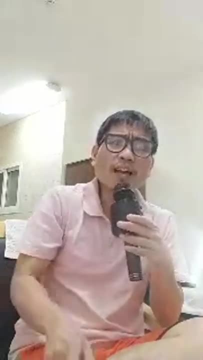 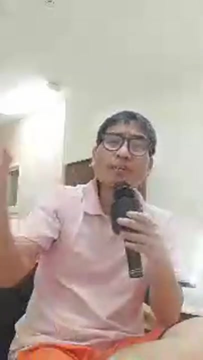 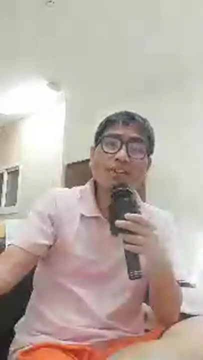 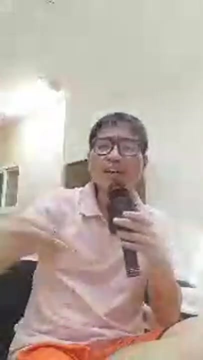 that's what we have always in. you know, in the process will always have bleed, bleed off the LED somewhere on the terminal of the pipe, something like that, and the other is the vent, ve and T vent or the bleed off, you know, opening. okay, because to give way for the vapor and for the liquid. 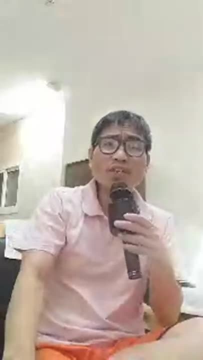 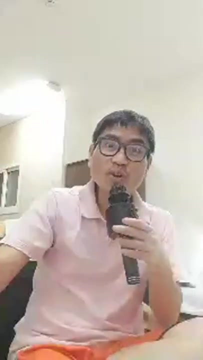 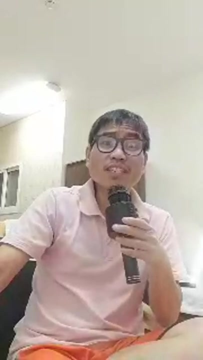 something like that, because if not, then it will build up pressure and just tend to see that your pipe will burst b-u-r-s-t. okay, and then it will crack somewhere along the way and it will explode, okay. so this is: we need to have vent, vent for the steam, and we also have 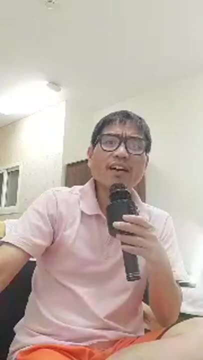 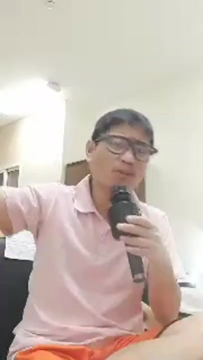 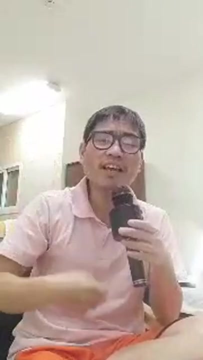 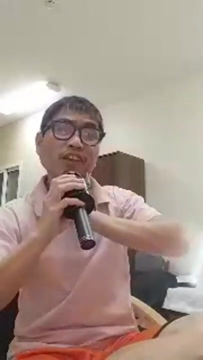 to bleed off the big led, the water, the moisture on the pipeline. it's gonna be on the end or it depends on the situation. where did they put that one? okay, okay, so during, like me, before i am working in the sabic. uh, you know something? affiliates or southern industries in saudi. 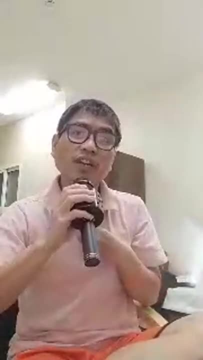 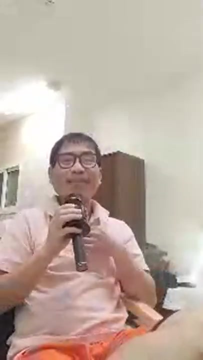 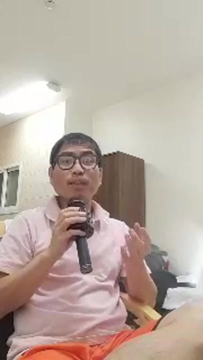 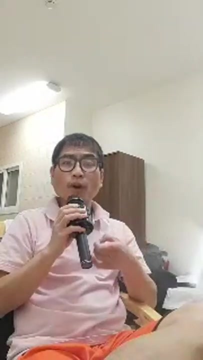 kaya petrochemical. i work there as an office engineer. okay, i am assigned in the uh olefin, my gosh chemicals- producing chemicals derived from petroleum. at the point, it is an industry that producing chemical products derived from petroleum. that's why their products are petrochemicals. 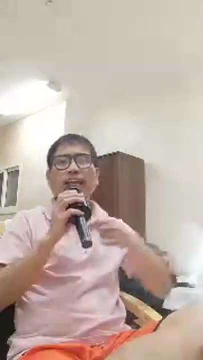 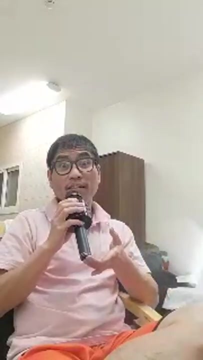 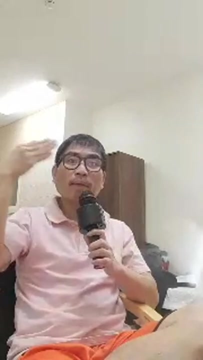 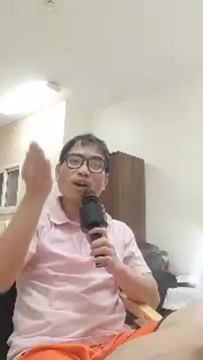 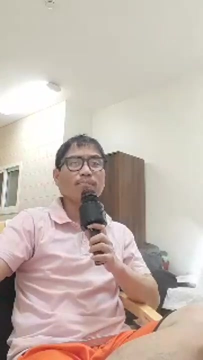 a combination of petroleum plus chemicals. petroleum is the raw material and the product will become petrochemicals. okay, combination of petroleum chemical. that's why petrochemical products. it's derived by crude oil and it's also undergoing fractional distillation. so this is now the second type of distillation. this is not simple. 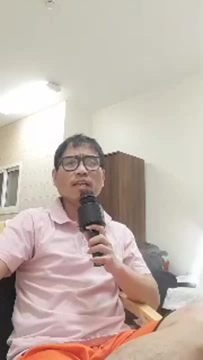 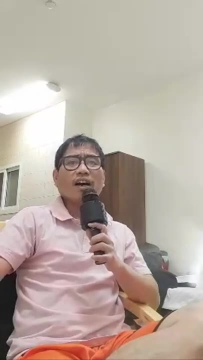 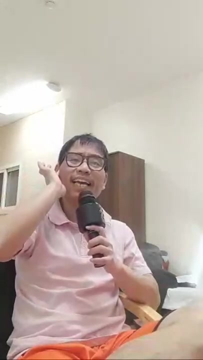 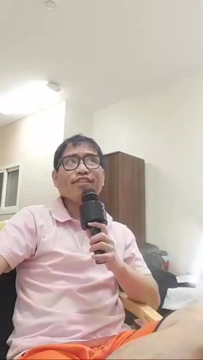 anymore, because you have to separate liquid to liquid, liquid to cast liquid with liquid, uh, done by fractional distillation. okay, oh, this will be applied in petroleum industry, something like that, in which your raw material is the crude oil and then it will produce a lot of multiple products useful to. 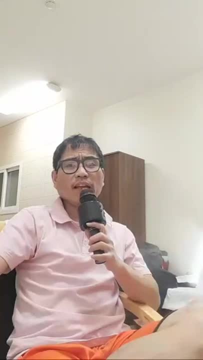 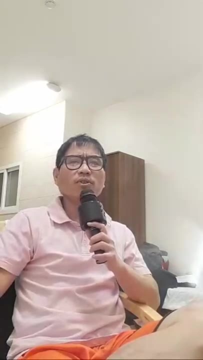 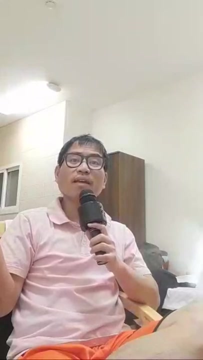 us, for example, it will produce. okay, as far as i could remember, it will produce. oh my gosh, stop knowledge between b i t u m i n: the black one that can be used in asphalting the road. okay, so this is also expensive, but this is produced by crude oil during the process. 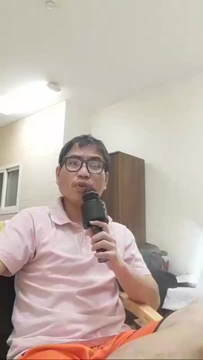 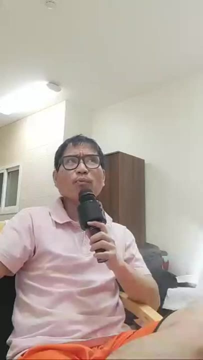 okay, and it will produce also diesel fuel to, you know, to fuel our cars, something like that, right, and then it will produce also petrol, gasoline, something like that, and also kerosene that we use in our home- it's a gas also- and then it will produce also. 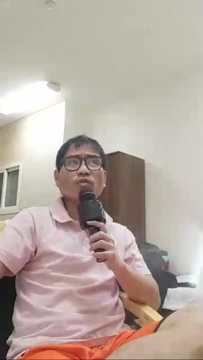 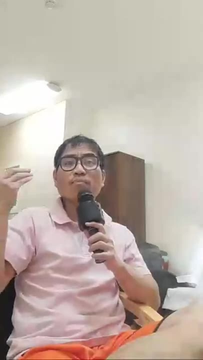 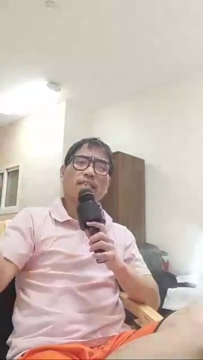 nafta. okay, nafta will produce also various products, for example naphthalene ball. okay, that we put in our toilet to remove the smell of the toilet. bad odor, so it's coming also from crude oil. look at the point. that's naphtha n-a-p-t-h-a. so nafta, kerosene, petroleum diesel fuel. 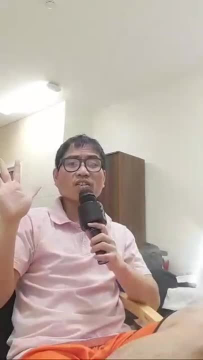 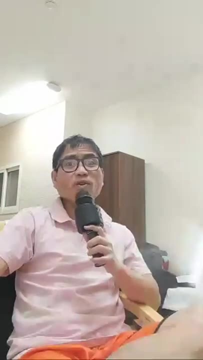 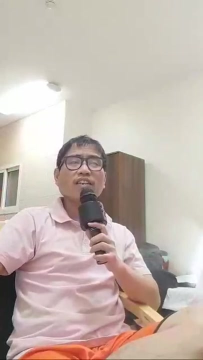 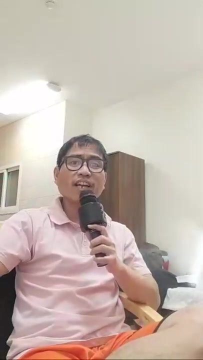 and bitumen. so these are all expensive products. comes from the raw material, crude oil. okay, and this is also used to power the plant, the factory, something like that, to run the different kind of electrical motor tabs, mechanical motor pads, so that we have power to produce electrical energy, something like that. so chemical energy converted. 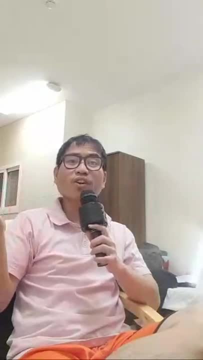 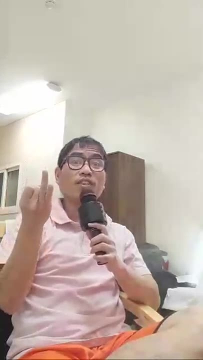 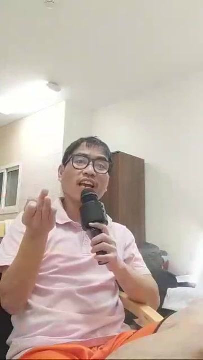 converted to light energy. imagine the role of a crude oil is: starting from chemical energy, converted to mechanical energy because it runs the motor pumps and whatever jojo, and then it converted to electrical energy because there's an electron slow in the path to produce power. and the last 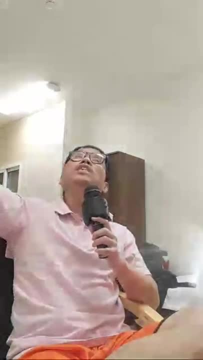 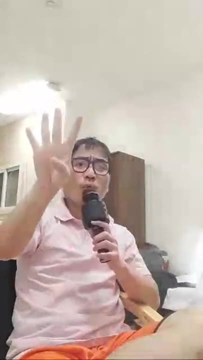 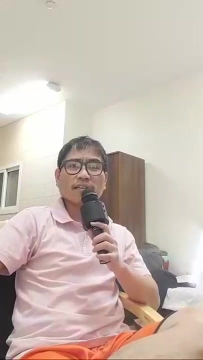 it will produce light, energy in which we see, in our homes, in our, you know, in our factories or whatever. so it will be four. for example, if the examinations will say like this: what are the four processes involved to produce a light? okay, so you have no clear idea. enumeration. 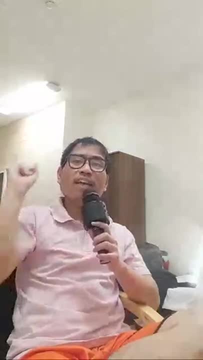 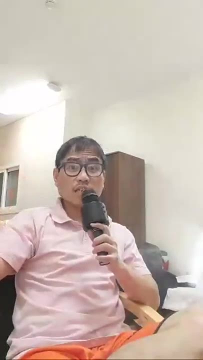 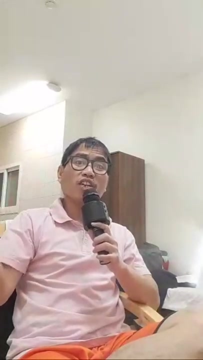 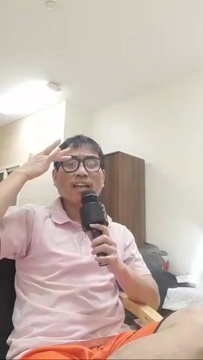 question: no, multiple choice. you will start with chemical energy, mechanical energy, electrical energy, light energy is the last. okay, you get the points. it is also the situation. because another thing also: it will produce sound energy at the last. okay, this also like the sound system, like that. okay, the instruments or whatever started with a chemical, always okay. 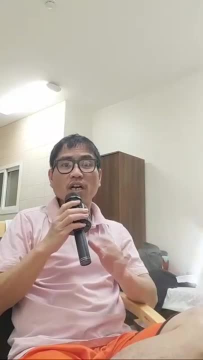 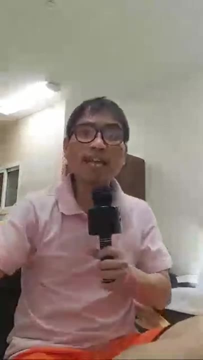 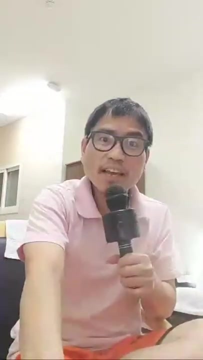 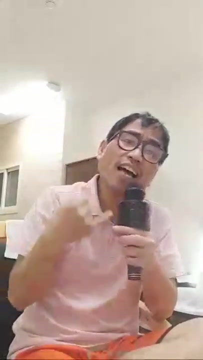 all materials in the planet earth are made of chemicals. okay, there's no escape, even water. water is a chemical composed of oxygen and hydrogen. okay, elements are chemicals already. okay, you get the point. so it's also a chemical energy. okay, so that is fractional distillation. again, it involves a condenser like that. it's also involving you know, uh, what? people just want the. 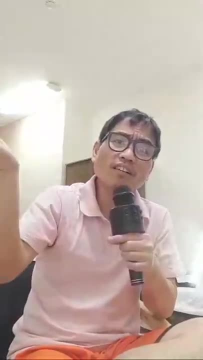 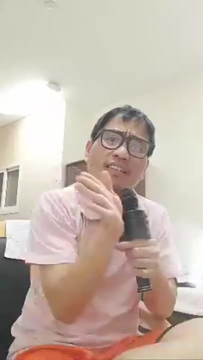 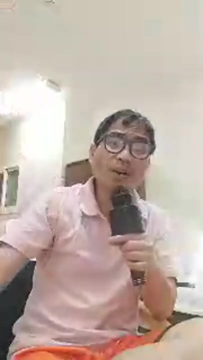 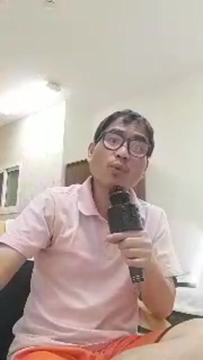 recoil okay, reboiler okay, in which the condenser will go there okay, and then the distillate will go there. now pump in the upper portion to the reflux- you know reflux condenser unit at the top to produce the overhead product. okay, as, because that's what we can remember- the reflux is the ratio of the you. 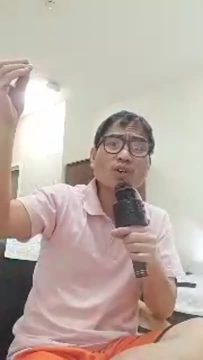 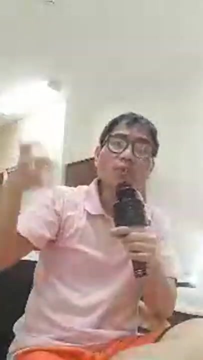 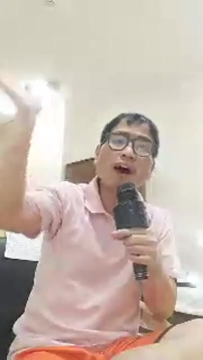 know, the final distillates right to the, the final distillates that will go back to the distillation column and the distillate also that can be withdrawn to the column. solution: call something like that an equilibrium room. okay, something like this. what would go out and then in? 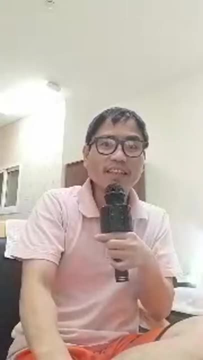 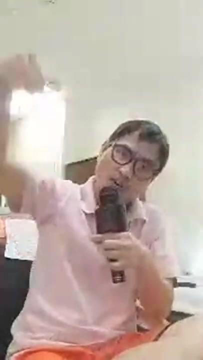 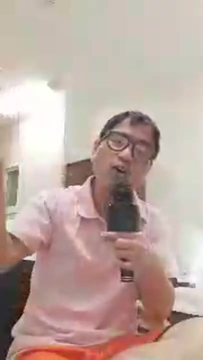 already will be applied, because there's a gravity, something like that: okay, liquid going down, okay, liquid is a downloading pressure going down and vapor will be the uploading, the upward pressure going up, and vapor will be collected, it collect and then it will produce, uh, a condensed liquid, something like that. 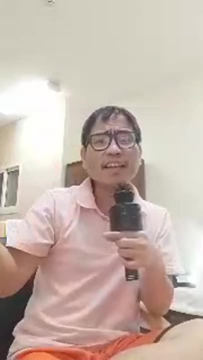 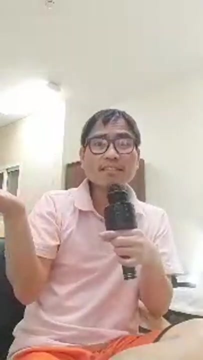 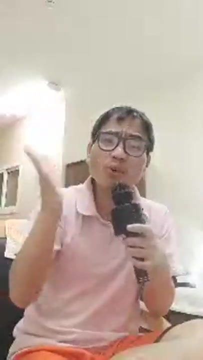 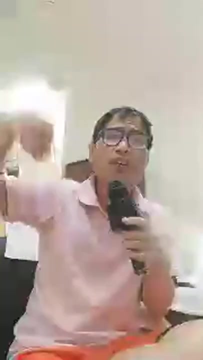 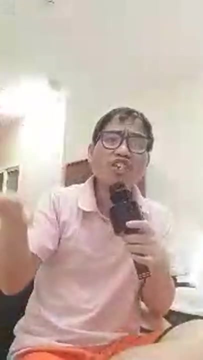 uh, condensed liquid is the distillates. um, okay, i just eliminated more on the vapor, state fishermen me and distillate more on the liquid product. um, because, as much of molecular weight or boiling point, I'm gonna ask, Okay, I will arrange it from large molecules or large boiling point or other molecules for the vapor. 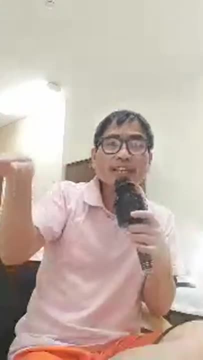 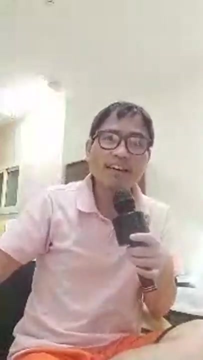 and thats it. okay, okay, okay, Okay. boiling point downward and then goes up Ang lighter na siya sa taas. Okay, of course, magpa-obos dyan ang lighter ang bugat. Okay, ganun siya, Okay, na ma-produce din siya. 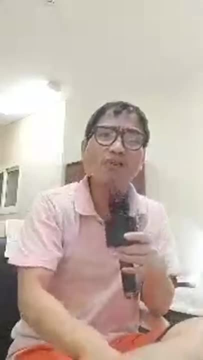 of once and mga fractional distillation ma-produce din siya of mga dodecane. Masabi ng dodecane sasabihin naman na dodecane dodecane class is 12 carbon. 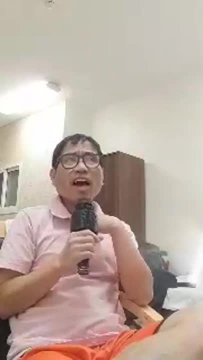 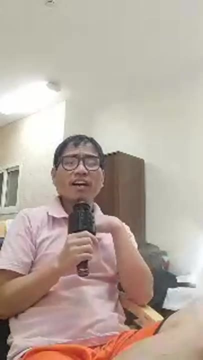 atoms siya. Okay, dodecane And then dodecane gravitation, yung mga ganun, in fairness. Okay, mayroon siyang mga 10, octa is 8.. Okay, nonane, kung nonane. 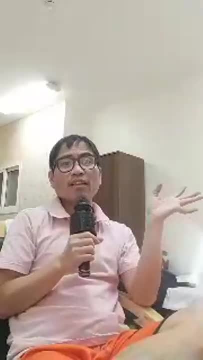 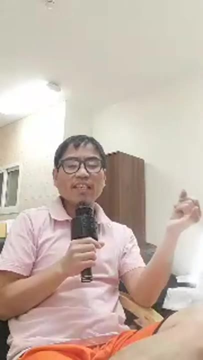 kay 9 siya, mga ganun, Octane kay 8.. Mga natin natin octane, mga natin siya ang gasoline, Okay, kung natin octane ako tay, nonane, Nonane, dodecane, Kung 12 siya. 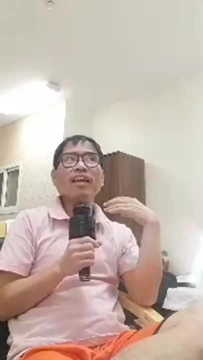 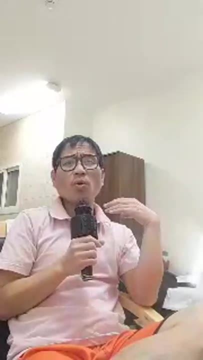 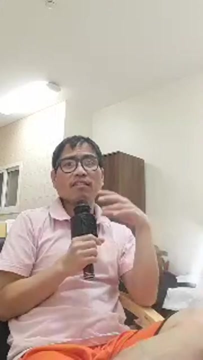 guys dodecane siya, Wow, ganun. And then dodecane is a large molecules, has a high boiling point, And then it will undergo thermal cracking to produce smaller molecules na siya, in which mabulu siya of butene and octane. Okay, ako may show. 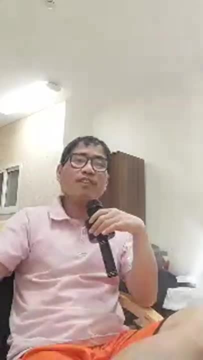 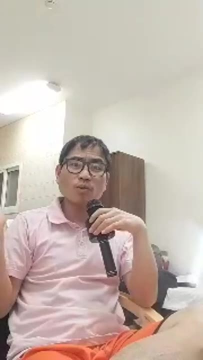 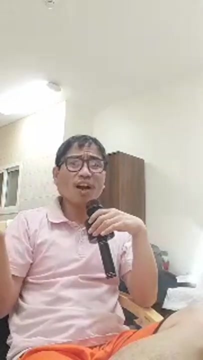 this also involves organic chemistry In physical separation processes. guys, naagin permi ang organic chemistry niya Ara Okay. and you should never forget the principles and foundations of organic chemistry, especially in petroleum, Because petroleum are really, you know, hydrocarbon really is studied by. 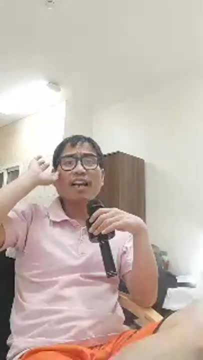 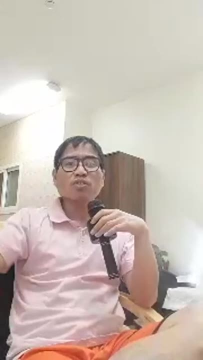 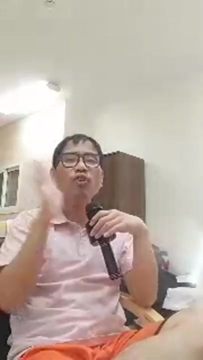 organic chemistry. Okay, lengthy or long chain of hydrocarbons, hydrogen atoms and carbon atoms attached to the, you know, to the band B-O-N-D banding. Okay, something like that, You get the point. Okay, ang kanong dodecane guys. 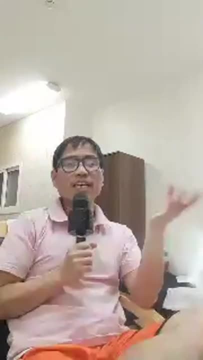 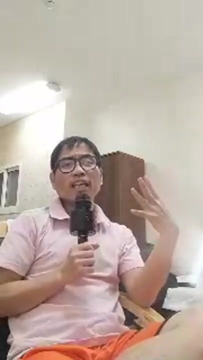 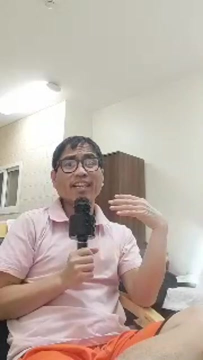 Diba Gigan siya sa fraction ng mag-destillation ka first, And then another process also. Okay, this is now the thermal cracking: Thermal cracking and catalytic cracking. And now this thermal cracking requires a very high temperature to manage to produce molecules. 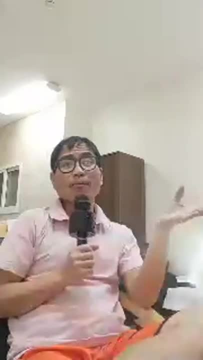 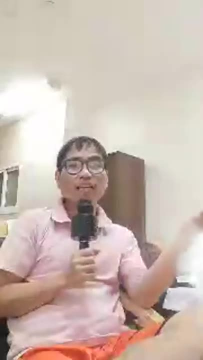 smaller molecules from large molecules to produce a lot of petrochemical products. right, As I mentioned, ako nagaw Coming from you know petroleum like that- Okay. for example, I have dodecane- Okay, so I have so many products will be produced that mga lower molecules. 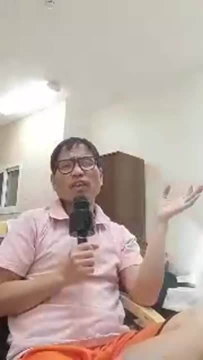 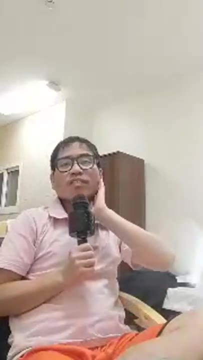 na lang siya, So dinina na siya. 12 carbon atoms It could be. there is octane, gasoline, okay, like that. So, in short, octane coming from dodecane, Charot, The gasoline we have. 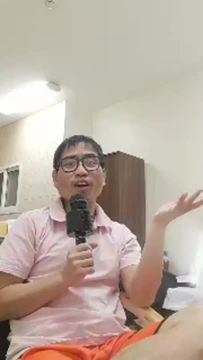 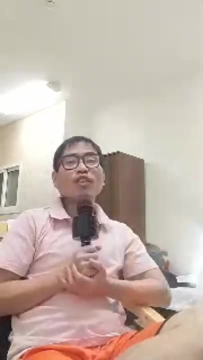 is coming from a very long chain of hydrocarbon known as dodecane. Okay, now, kung makalimot ka sa formula, Limot ba ya ako In monod, yung timan anak akong tulungka pattern chemical formula sa organic Okay. 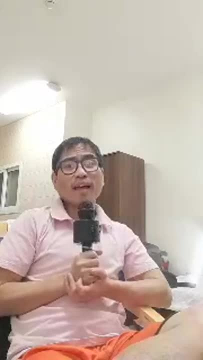 now I will discuss to you: CNH2N plus 2 is the ENE family. Okay, single band. Okay Now CNH2N: okay, mga ganun-ganun. siya Mono na siya ang double band. Okay, double band. 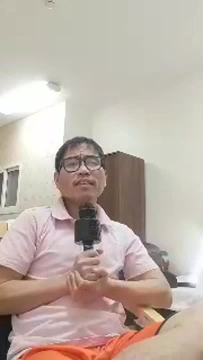 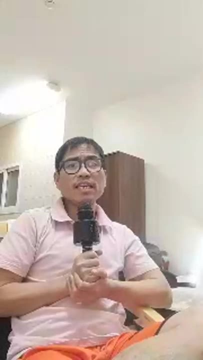 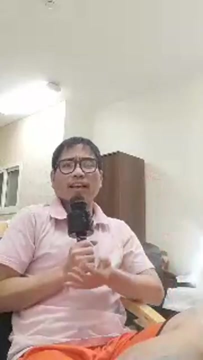 siya Okay, And then H2N minus 2 will be our triple band na nag-ent siya sa Y and E. Okay, so this is basically organic and vegetable. Alkane, alkene, alkane, Ganon- Okay, acetylene, Ganon. Acetylene is. 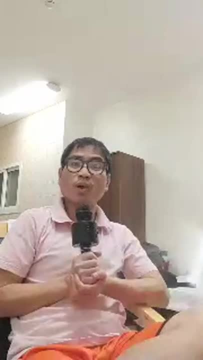 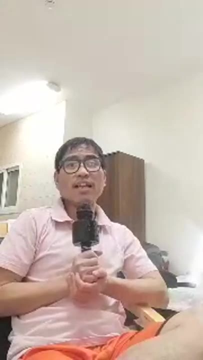 a double band, The, you know the gas cylinders we have in welding operations or gas welding operations. So that is a double band. Okay, E and E, N's E and E. So acetylene is a double band. So acetylene means two carbon atoms, Something like that. Okay, And then the rest. 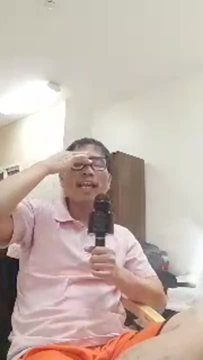 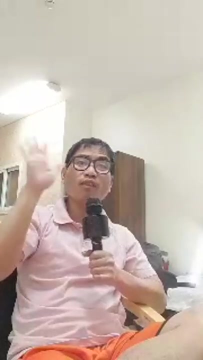 will follow. The hydrogen will be dependent on the formula: na siya, Okay. The small letter N, guys, is the number of atoms. Substitute the number of atoms there and bingo, you can have the exact formula of a hydrocarbon, For example. I will say butane, there are four. 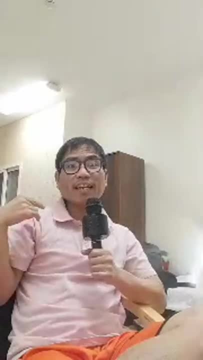 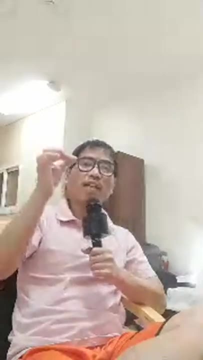 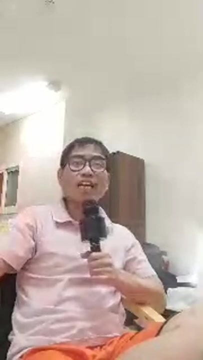 carbon atoms, So butane di ba E and E, ang last three letters, So that is CNH2N plus 2.. Substitute the four in N, So CN, C4H2N, So 2 times 4A, Like that Plus 2.. So that is C4H10.. So C4H10 is the formula. 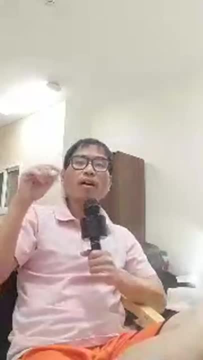 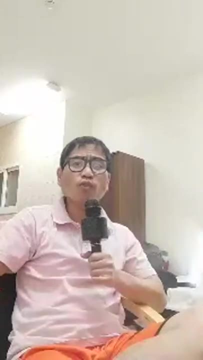 for butane. Ang imo tema na ng formula rin siya nga katokong giingon, tulok ka buo. Okay So, bisag pila pa naka million-million di ha. isubstitute din mong carbon atom masolve. 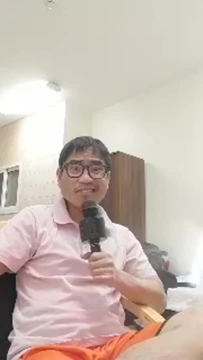 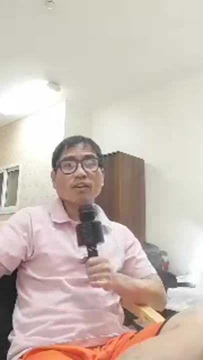 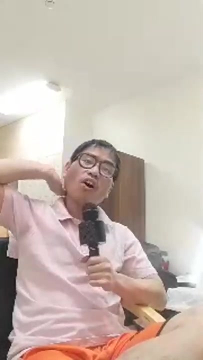 din mong siya formula sa organic compound. Okay, guys Like that. For example, I have 100 atoms of carbon, So I can still compute what organic compound is that? How, Having 100 atoms of carbon, Okay, Ganun siya. So that is for oil refining, For crude oil. 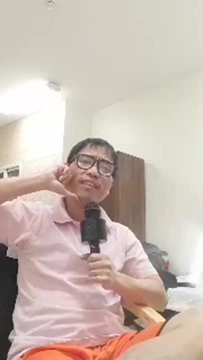 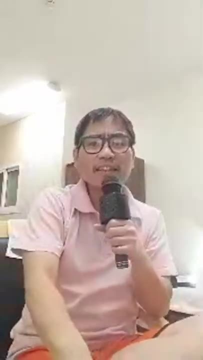 refining, Something like that. Okay, You need to see if that is crude oil raw material, pa siya. Okay, It's not yet the product. Do you get the point? It's gonna be like that. So we need to have examples for distillation, Of course, if we have the types of distillation. 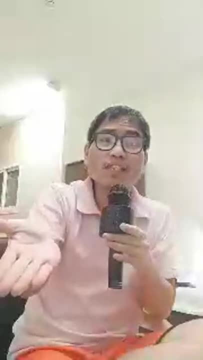 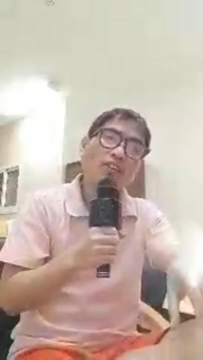 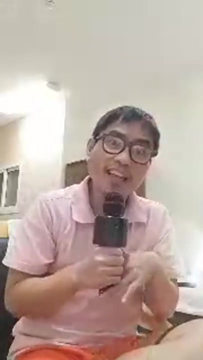 we need also to have examples of distillation. So what are those examples of distillation? For example, apart from oil for oil refining, isa naman siya example, right? So making liquefied gas from air. Okay, Air, you know. 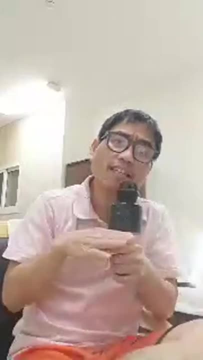 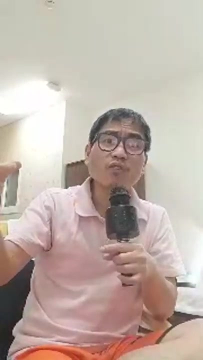 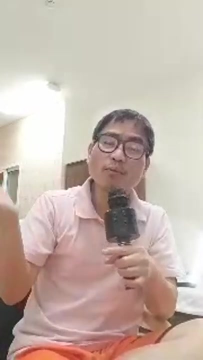 we capture the air atmosphere and we can produce gas. liquefied gas, meaning in liquid state. Okay, Because liquefied gas man siya, So meaning adjective added to a noun. We describe what kind of gas is that that is liquefied, so meaning the product is liquid, not a gas. okay, you get the point. 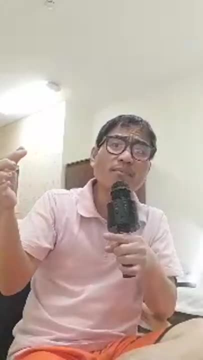 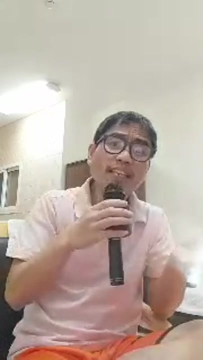 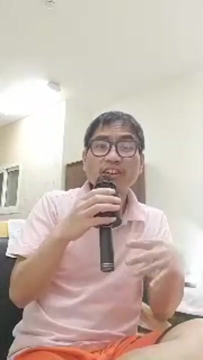 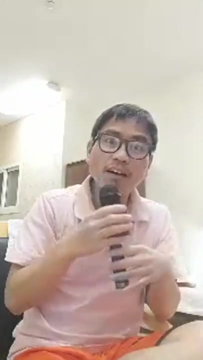 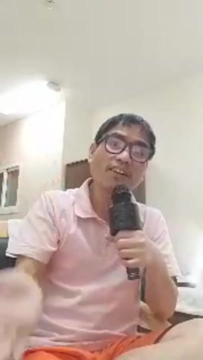 because this is a term: gas man. okay, so liquefied liquid. okay, like a professional singer, so singer, that is professional, just like liquefied, cast a gas that is liquid, liquid, informed. okay, just like that in english to describe something, to describe a noun, that is an adjective, right? so it's gonna be like that, also liquefied. 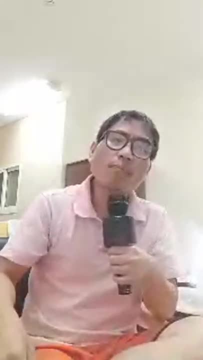 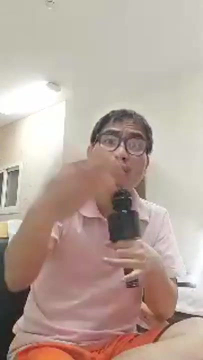 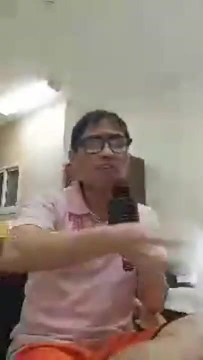 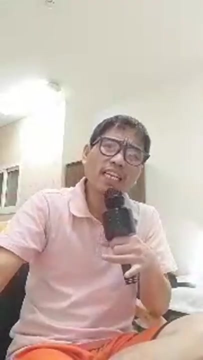 cast: okay. so making liquefied gas from air: okay. and then we have also purification of water or alcohol. purification of alcohol and purification of water also, for example, to produce wilkins product the most. the purified distilled water that we buy in the market, okay, distilled, almost pure water. so we remove the. 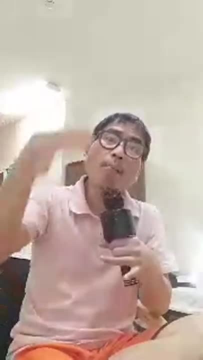 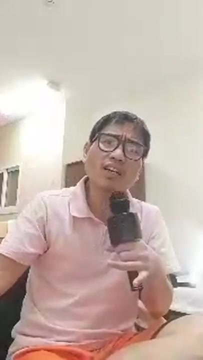 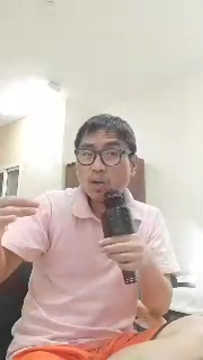 minerals. for that it undergoes distillation process, so it is purification of water, okay. and then we have also purification of alcohol, starting from a very large carbon atoms of alcohol and then you break that down to a lower number of carbon atoms of alcohol, something like that. okay, so it's gonna be methanol. 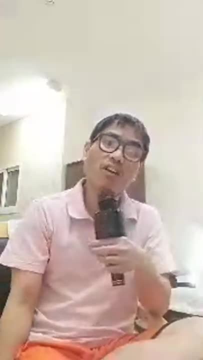 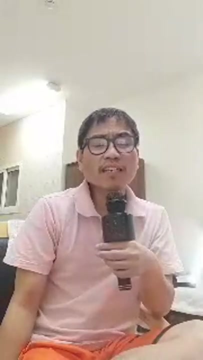 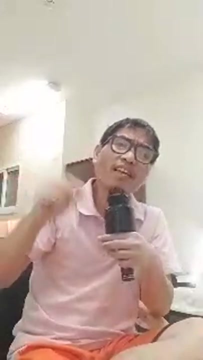 or ethanol right. the simplest form of alcohol is methanol, right. second ethanol, it will follow the term methanol, ethanol, propanol, butanol, propanol, like that. follow also the sequence of the prefects in algebra: okay, like that. okay, if three, if four, if five, if six, hept lineage. 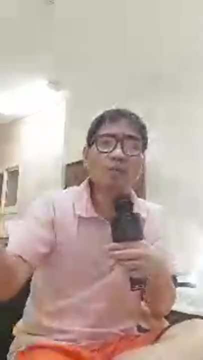 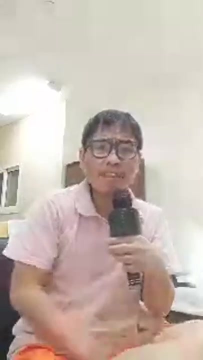 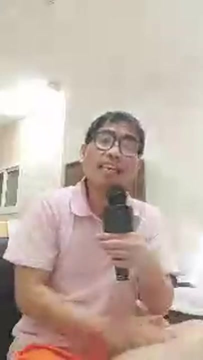 okay, you get the point. just follow that sequence also. okay, the same thing. okay, like that. okay, so that is gonna be like that. what else? the most important one that is going to be like that? what else? the most important one in the producing of drinking water? also, this is desalination. we need to remove the salt. 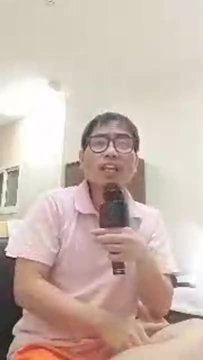 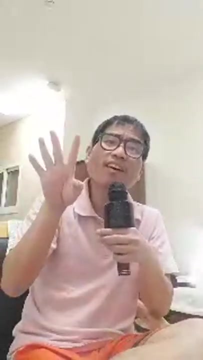 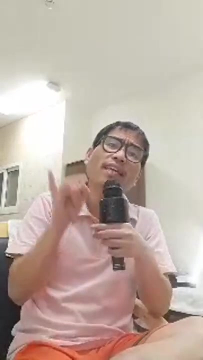 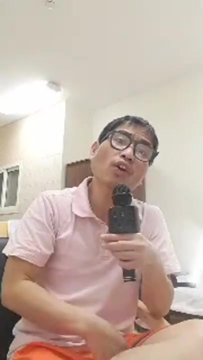 okay, from seawater to produce drinking water. this is also example of distillation. actually there's a lot. this is only the four basics. okay, crude oil refining. okay, purification of alcohol or water. okay, making liquefied gases from air and then desalination process: from seawater or sea to 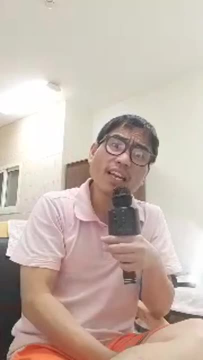 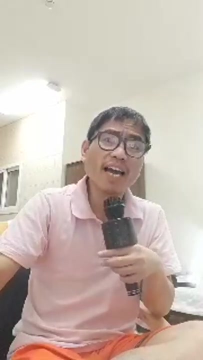 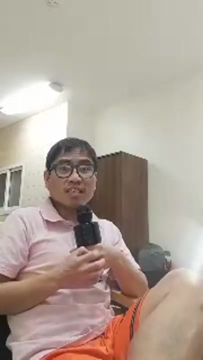 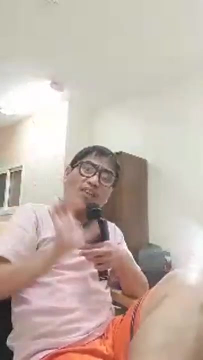 drinking water, okay, like that. but this is, you know, this is expensive, because how many you know distillation units you'll be able to buy. that's why this is not really practiced most of the time. because we have no reverse osmosis, okay, we need to get the seawater and pass to the semi-permeable membrane, a filter, because this 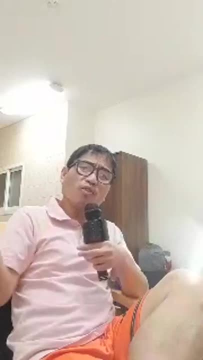 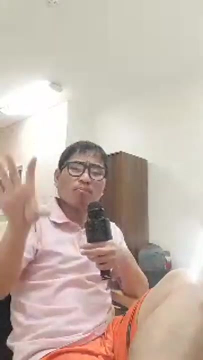 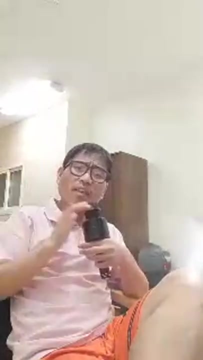 is more, not too much costly compared to the distillation columns. this is the solution. columns are very costly compared to the equipment for the reverse osmosis, in which we have the smaller one. like that, that's not too expensive, okay, and then your product also will be more. 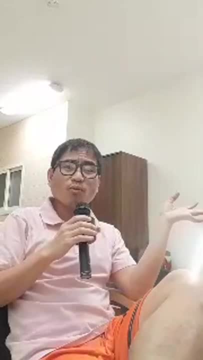 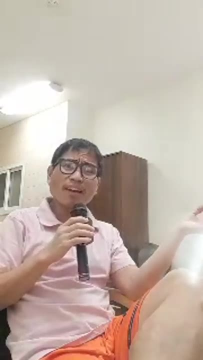 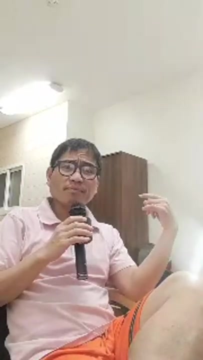 compared to that. you know how many distillation column you put in the laboratory just to okay, just to get the seawater and then convert that to drinking water. right, it's like not inagical. it could still be possible, but not practical. okay, the costs are very high. okay, compared to just having the reverse osmosis. 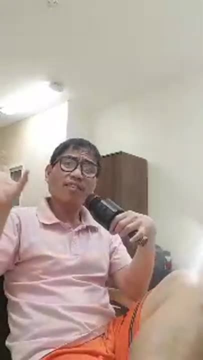 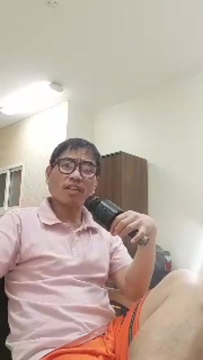 or shall we say the normal filtration only, such as water treatment, water refilling station, and so it's just like that, okay, in which not so much expensive business today in producing drinking water, and then you have the water analysis like this to take the parameters of water. it's just like that.